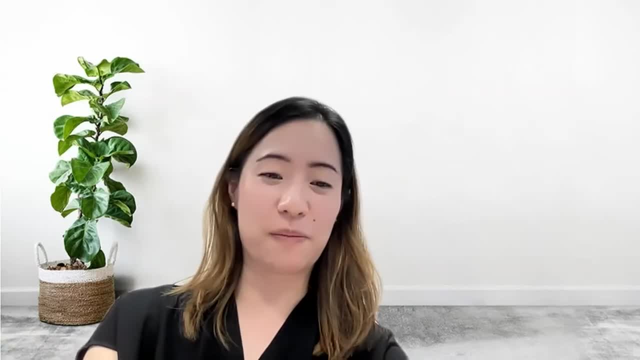 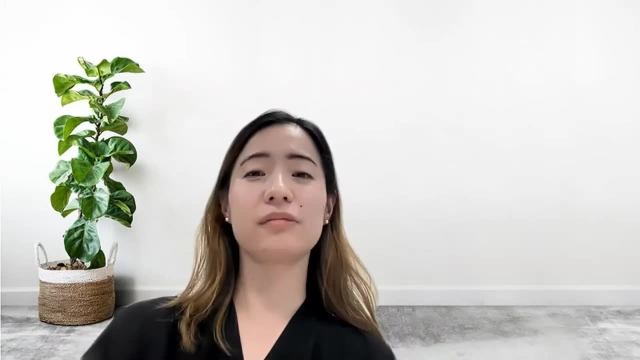 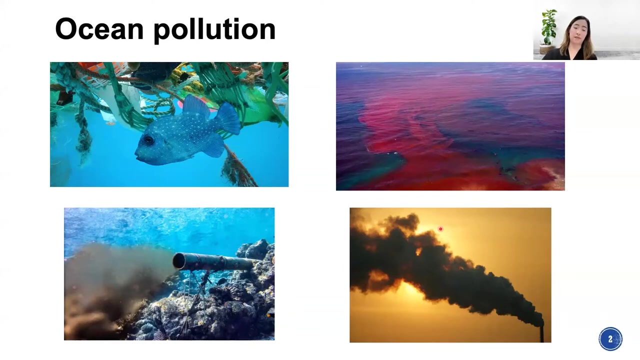 on the Zoom and especially in person. So I'm going back to my slides. So today we're talking about ocean pollution. So when you think about ocean pollution, there are many types of pollution. So now you can see the photos, especially people on the Zoom. The left is the. you know the fish entangled in this like 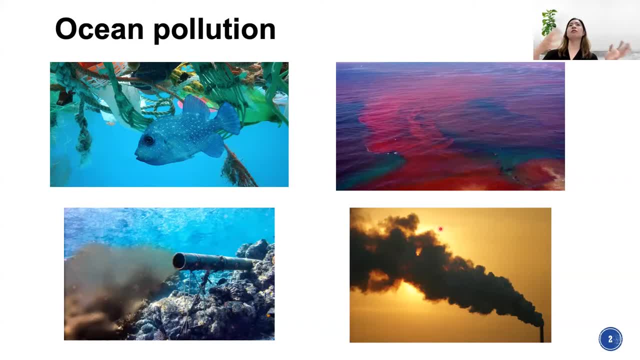 marine debris, The right is harmful algal blooms. So these are physical, biological type of pollution. So below these two they are chemical pollution. So chemicals: there are lots of kinds of chemicals in the ocean, As visible as the other two, because you know when you look at the water you basically can't tell. 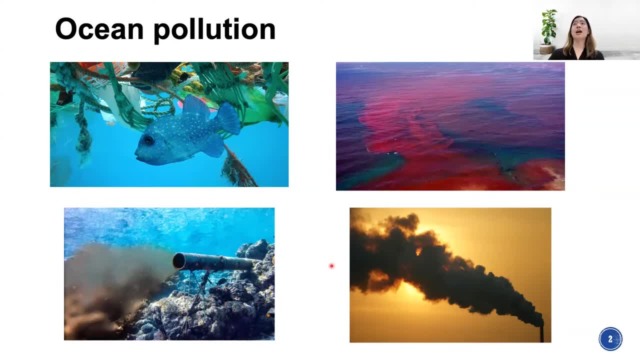 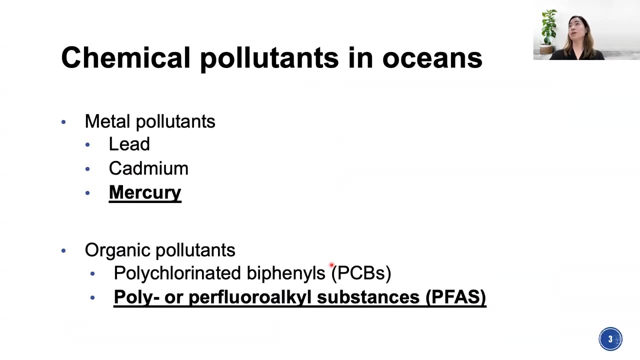 what are they and how much are they? But they are actually very relevant to ecosystem and human health And hopefully by the end of this talk I will convince you about that point. So there are also many types of pollutants- chemical pollutants- in the ocean. So I basically 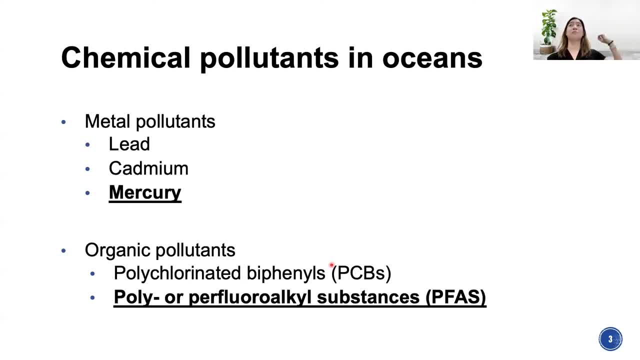 kind of broadly separate them into two types. One is metal, or we call it metal, and the other is inorganic pollutants. The second is organic pollutants. So the metal pollutants are usually, you know, the common ones you will hear is like lead, cadmium, mercury, And today I use mercury as an 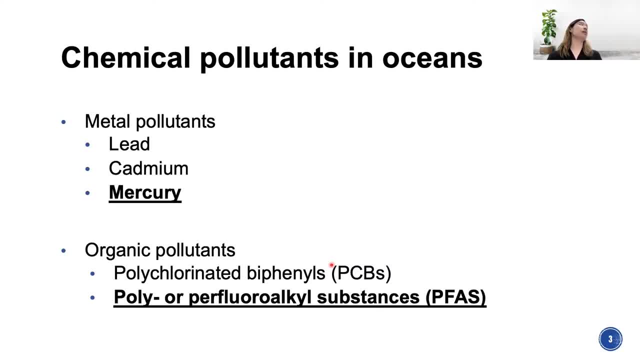 example, because I think it's just really interesting and relevant to our daily life- And for organic pollutants- you probably hear about polychlorinated biofennels, so in short, PCBs, And I will actually focus on emergent contaminants, which is kind of a new thing, that as the long name. 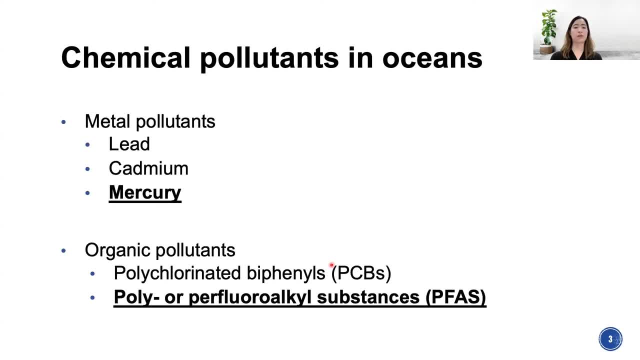 is polyperfluoroalkyl substance, so in short, PFAS. So that's something we just started kind of knowing more and more about that and draw lots of attention. You probably have heard from news or watched the news about it, but I think it's really interesting And I think it's really 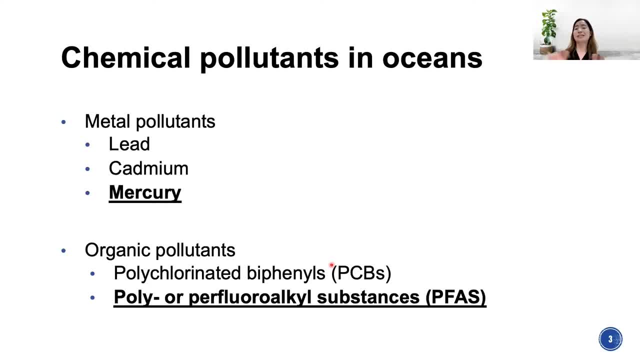 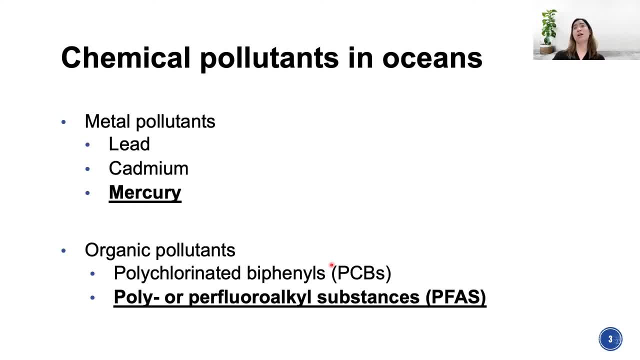 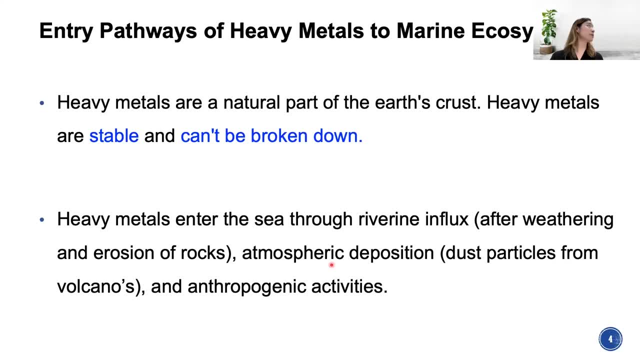 the meantime I will talk about this is kind of particularly interesting topic in this area, like Delmava area as well. So first of all let's talk about metals. So metals- very different from most of organic chemicals, Metals are a natural part of Earth's crust, So they are natural. 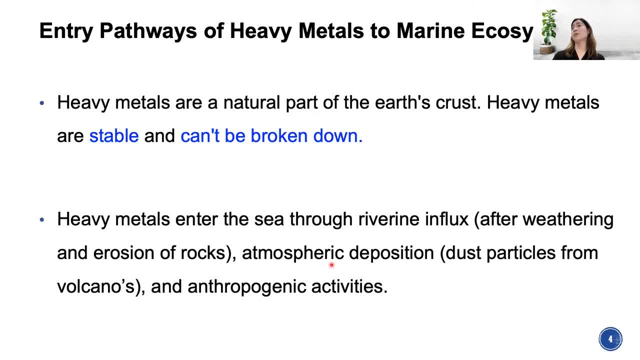 the heavy metals are. most of them are very stable, so once we extract and emit it to the environment, they can't be broken down. they just there and normally the the speed. you know, we, we have them as like a net. we emit them from natural sources, so volcanic eruption or weathering, these ones are. 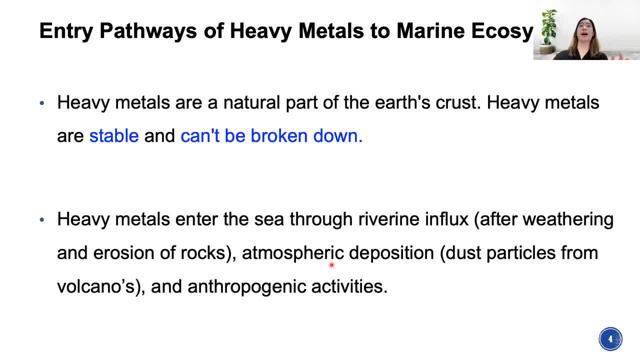 kind of in balance with the speed that we cycle that metals back. but anthropogenic activities really disrupt this biogeochemical cycles. in other words, we extract and input way too much heavy metals into the environment then the months that they can be cycled back. so when we talk about heavy metals, one thing i want to point out is they're- they're not all toxic. 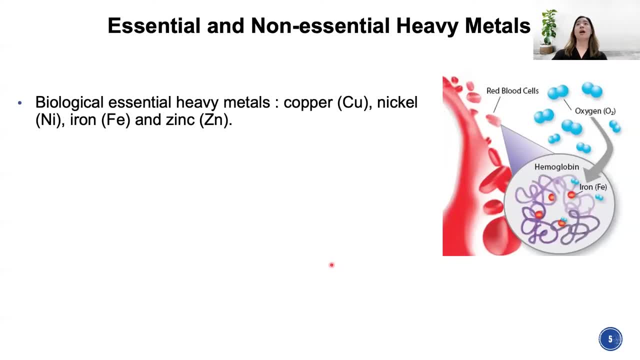 there are ones that are biological essential. so, for example, copper, iron and zinc, and the picture on the right and you can show you the iron is a very important element for hemoglobin, right. so if you have too low level you'll get anemia. so that's essential heavy metals, what we usually talk about heavy. 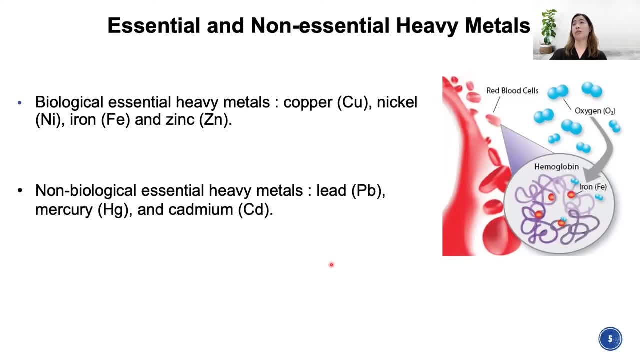 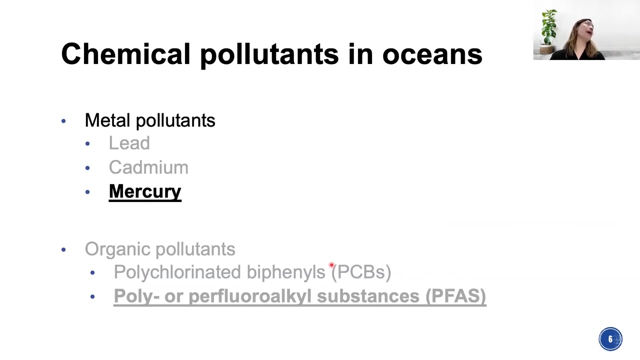 metal pollutants are these non-biological essential heavy metals. so these ones are. really. we don't need any of them in our body in order to maintain a normal biological functions, so any of them in your body is kind of extra and not necessary. so here today i focus on one type of metals that i have studied for a while. 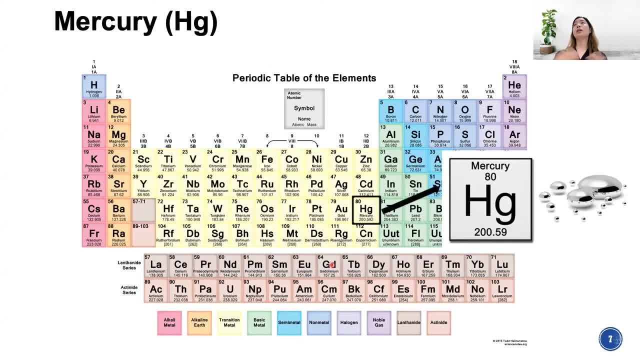 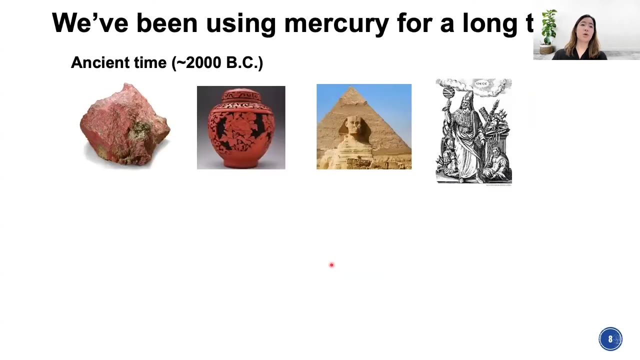 which is mercury. so if you look at mercury in the periodic table, they are definitely a kind of heavy elements and they are the only element of metal that are liquid at room temperature. so that's very special. as you know, when the metals the fact that we have been using mercury for really long time, so lots of time- we call mercury 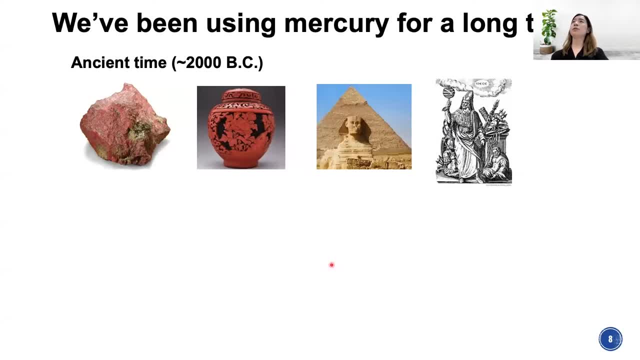 as a lexy, pollutants, so the mercury as other heavy metals, they are naturally occurring. so the left, the first figure, this: this picture shows that the, the rock that contains lots of mercury, and the sulfur, is called cinnabar. so if you want to mine mercury, these are the things we're going for, and the the red ones are where the mercury is. 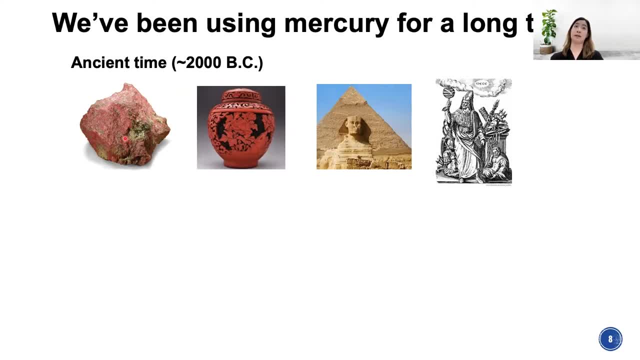 so mercury sulfide actually is a good pigment. that's why people have been using it as like a pigmentation and painting for a while- that's mostly kind of a really early time- and they also have been used so have been found to be a very important element of mercury in the DNA and the 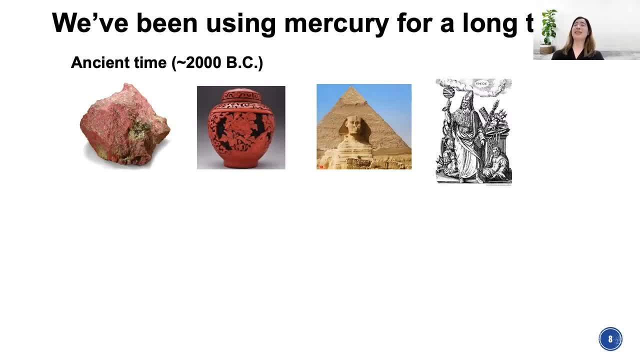 found in lots of like Asian tomb. So I believe, like people use it as like a symbolic river in you know, in these tomb And if you look at the Greek history, it had been used as for both, as like poison and the medicine. 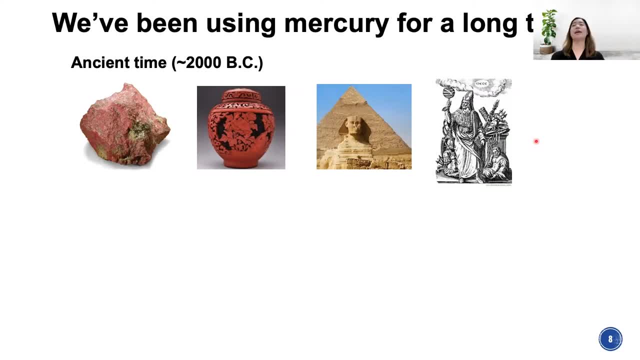 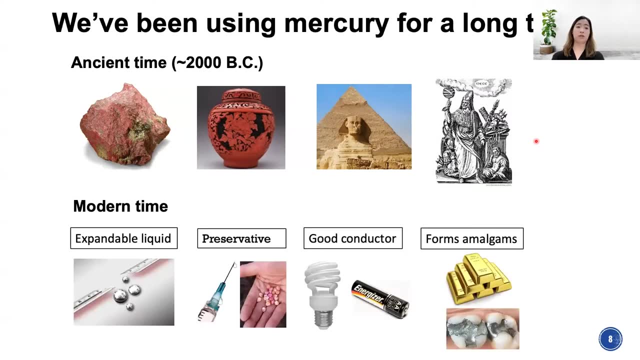 So that's really Asian time. then you know from history we know that had been used. but in modern time actually it's being used even in a wider application. So if you're older or as old as I am, you probably still remember that we used to use mercury. 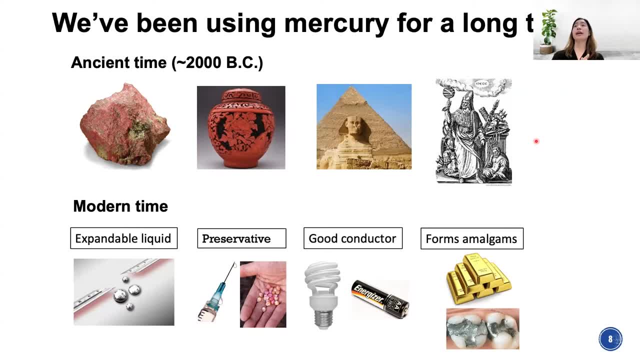 in thermometer, in barometer, because mercury expand quite a bit under a higher temperature, right. So it's actually really useful property. So that's why I mean we adopted it. we use it in the product Nowadays most of the mercury in thermometer. 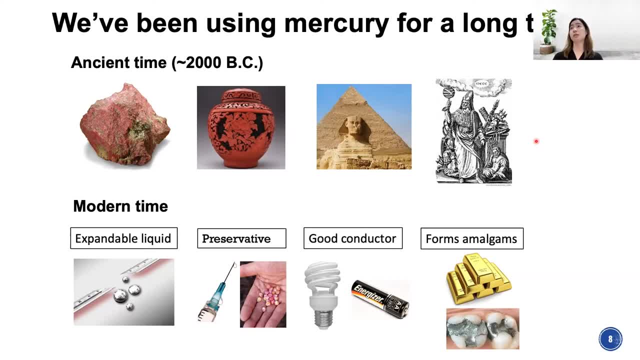 that this kind of use has been phased out in United States And then in general globally, So you probably wouldn't see this anymore. but I mean, I remember when I was little- you know that's something- my parents checked if I have fever or not. 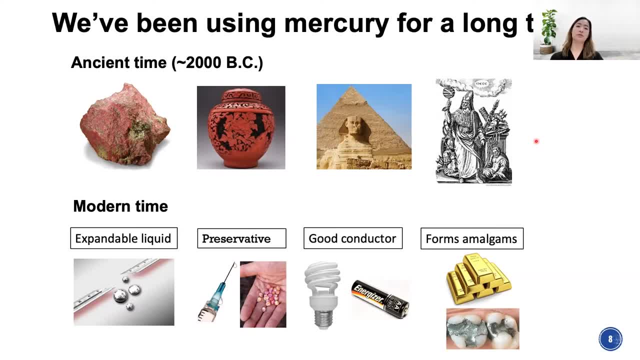 So the second one, so mercury. the inorganic form is very good antifungal and bacteria growth, So they have been used as a preservatives in lots of medicine, So that's quite common thing as well. They also are very good conductor. 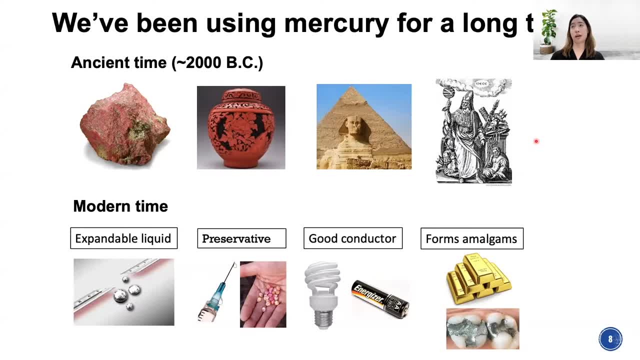 So lots of fluorescent bulbs and the batteries have mercury. As I said, lots of mercury containing products are phased out nowadays in United States. But if you go to store lots of battery now actually say mercury free because they used to be not mercury free. 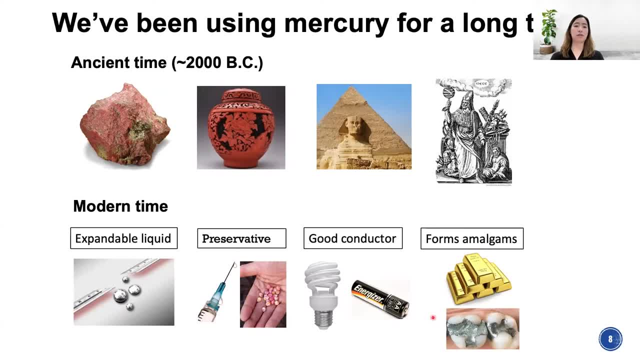 So the fourth one, the function that mercury has is- which is really important- it forms amalgams, So in other words they can bind and kind of make the kind of dissolve these other metals really well. So that's why it's widely used in silver and gold mining. 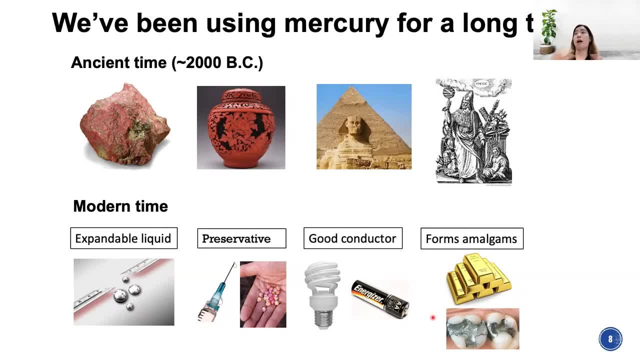 So that's what people did is, if they find some rocks that potentially have gold and then they put them in a pan, then they pour mercury- liquid mercury- into these things, then the mercury will extract these gold and silver from the rock And they form this kind of amalgam. 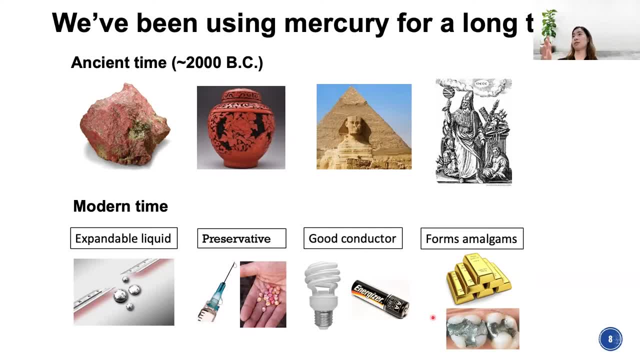 And then you kind of filter out the rocks that useless for you anymore. And then you have this mercury gold or mercury silver soup And what they do, because people want gold and silver. so they heat it up and mercury evaporate to the atmosphere. 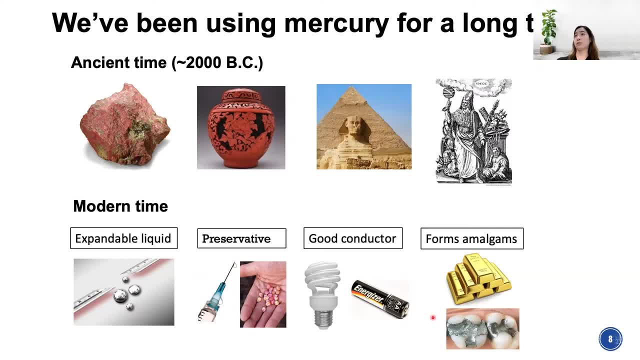 And the leftover is gold or silver or whichever other metals that they like to have. So that's been widely used as well, And still actually lots of artists and gold miners are using this tool And the last one- it's the same thing- that they 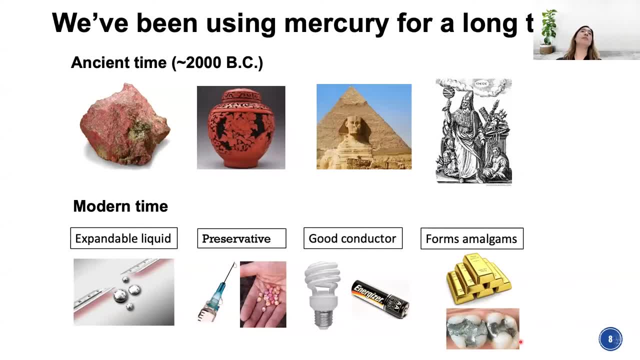 because they form really good amalgam with dental filling materials. So they actually mercury existing lots of dental filling. I guess I phased out probably a decade ago, but still I mean in lots of people's mouths. So if we look, take a look at you know. 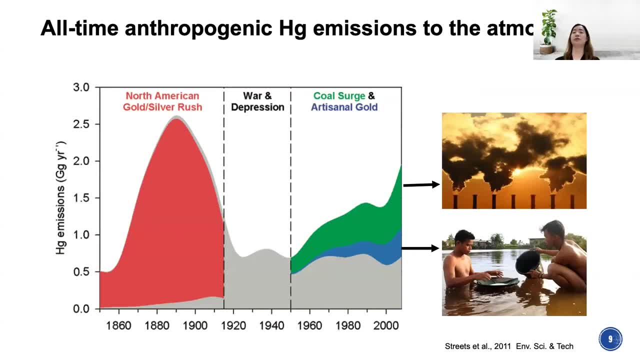 all time anthropogenic mercury emissions to the atmosphere. as I mentioned that it has been widely used in gold and silver extraction. So the in 1800, that the North America gold silver run has emitted large amount of mercury to the environment. Then we have relatively quiet time for the wall. 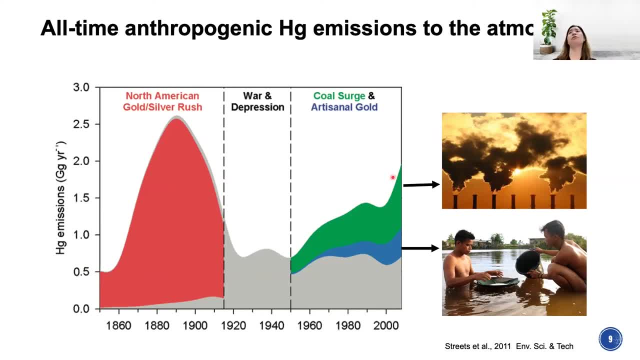 Then nowadays it's really the coal combustion or in general, fossil fuel. So the coal combustion and the artisanal gold mining that are contributing lots of mercury into the atmosphere. So the coal, the reason the coal and other fossil fuel has mercury. remember mercury is natural occurring in the earth's crust. 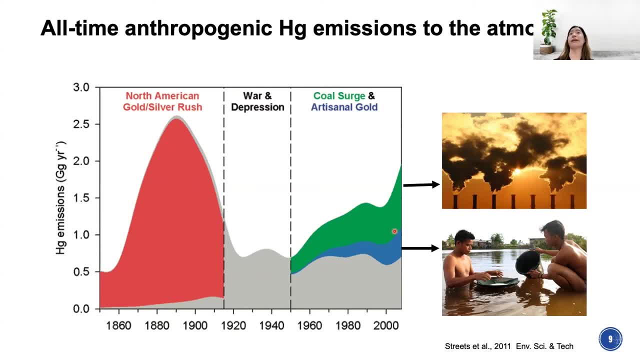 So anything we burn that we get from the earth's crust that has mercury inside. So that is these ones are that we emitted mercury, basically unintentionally, because the purpose is using other things. You know, you want energy or you want to get gold. 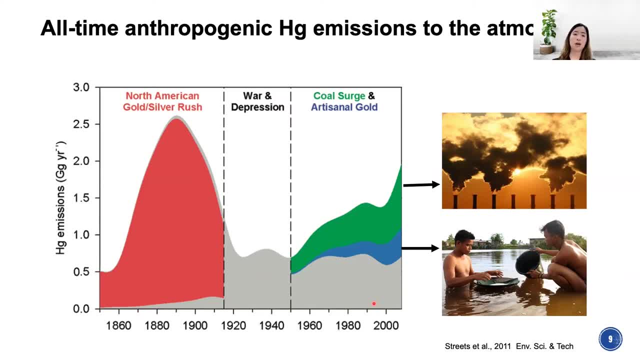 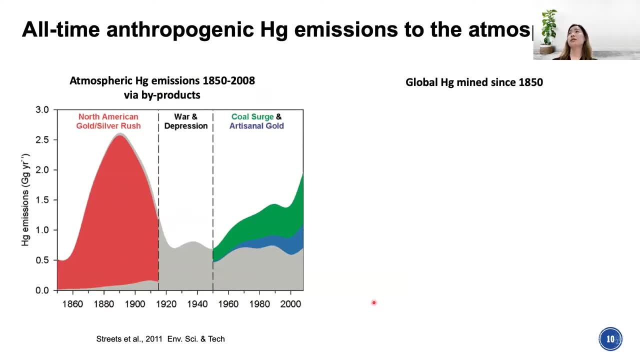 but unintentionally emitted lots of mercury into the atmosphere. So if we compare this mount with the global mercury that mined since 1850s, so this whole you know peak and the shaded area, they actually only count a very small amount of the global mercury mined. 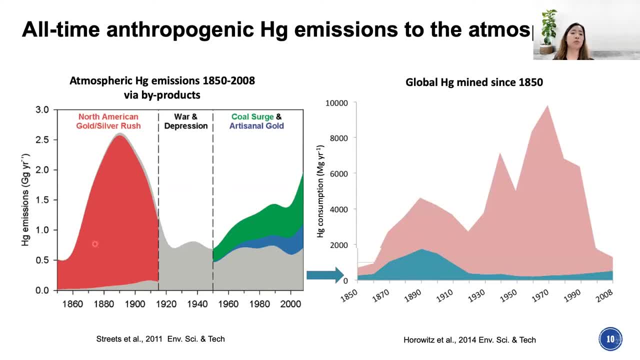 since that time. So this is the. this whole chart only equals to the small area of like sun shaded area And this whole pink area. that means we mined. So we use the mercury somewhere. It has not been emitted to the atmosphere. 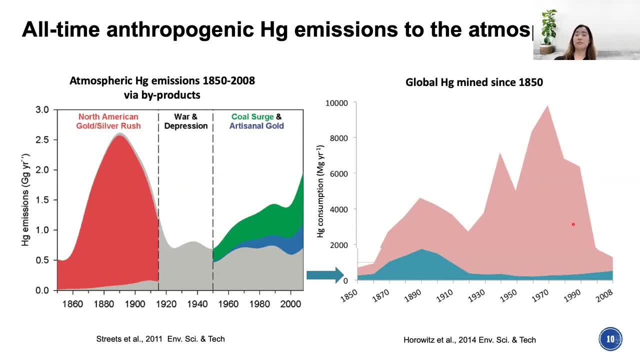 Who can guess where they are now? So they are in the commercial process, They are in the commercial products we talk about, And so you can imagine lots of them either in the landfill, if they already, you know, been buried and recycled, or I mean still in your household. 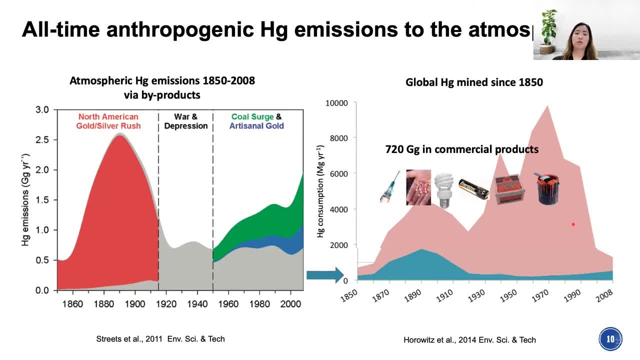 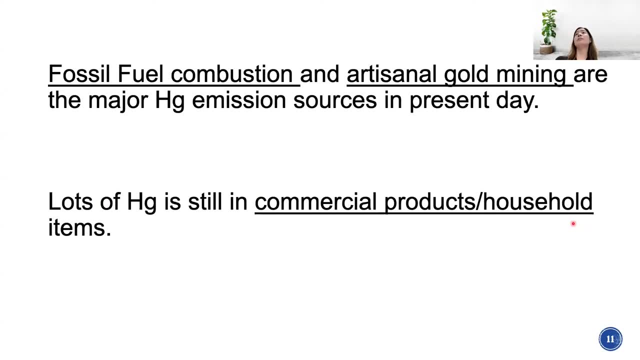 and this will be a long lasting problem, right? So just to kind of summarize what I said just now, that fossil fuel combustion and artisanal gold mining are the major two mercury emission sources in present day, and a lot of mercury still in the commercial products. 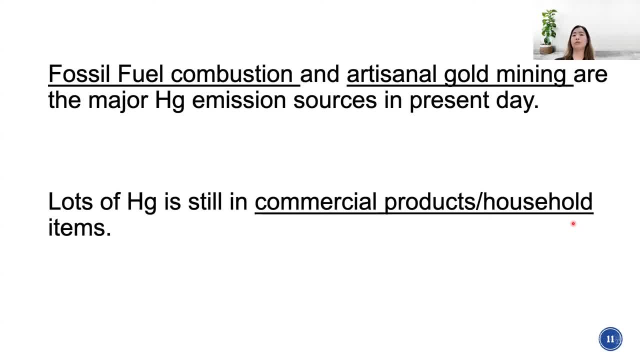 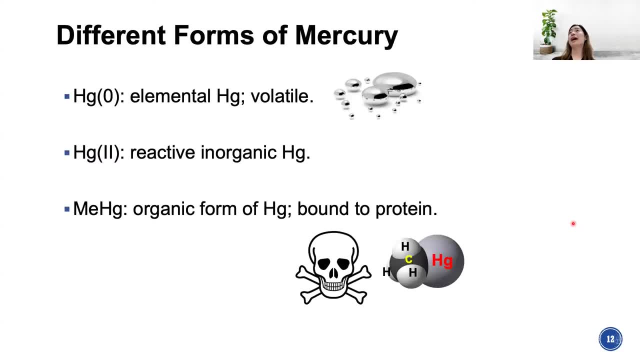 and the household items And before jumping into you know how they're relevant to, like a mercury in the ocean. we have to talk about different form of mercury because mercury actually quite complicated in terms of their biogeochemistry. Mercury has major, like three major forms. 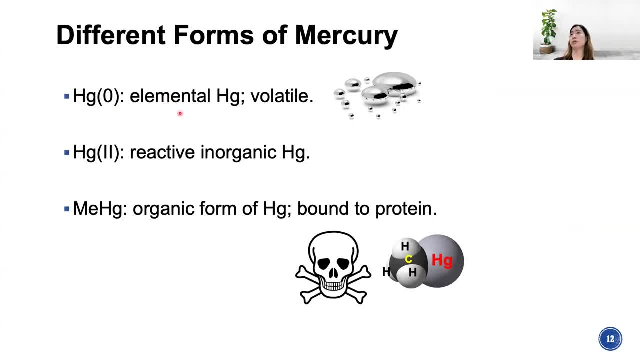 One is elemental mercury, So this one is volatile And they also have an oxidized form, mercury. two plus This is a reactive form, And then this is a methylmercury, which is the organic form of mercury. This one is much more toxic than the other two. 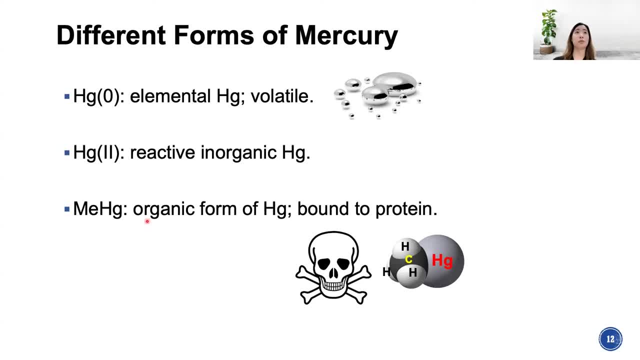 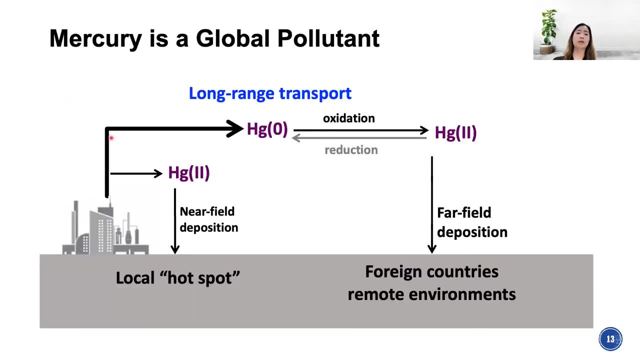 And unfortunately this is the dominant form in our seafood. So the mercury usually are emitted, say, from coal combustion or gold mining facility, that to the atmosphere. as most of them are elemental mercury so they're volatile, They actually can be circled around the globe. 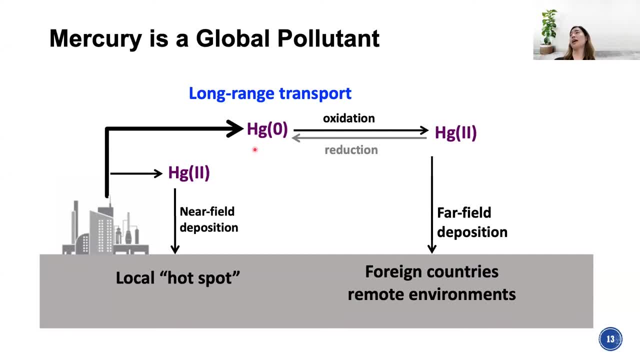 for a really long time. So if you test like mercury in the atmosphere in most of place it's basically a mercury from all around the world. It's not, you know, it's really not from a local spot. They have really long resident time in the air. 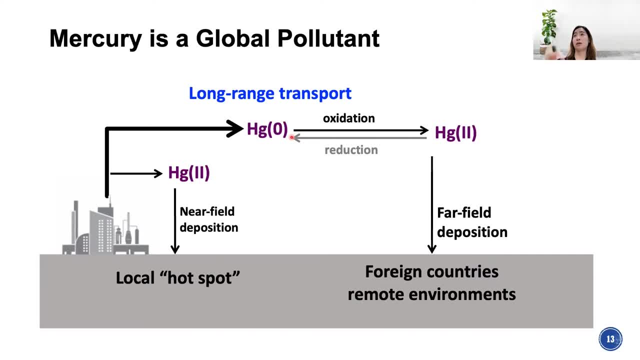 So this partial of this mercury zero elemental mercury will be oxidized in high troposphere to mercury two plus. This is the reactive form that could be bring down by precipitation. The mercury zero actually is not. That's why they can circle in the air for such a long time. 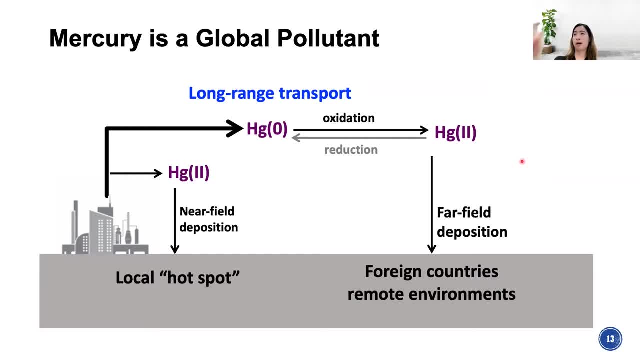 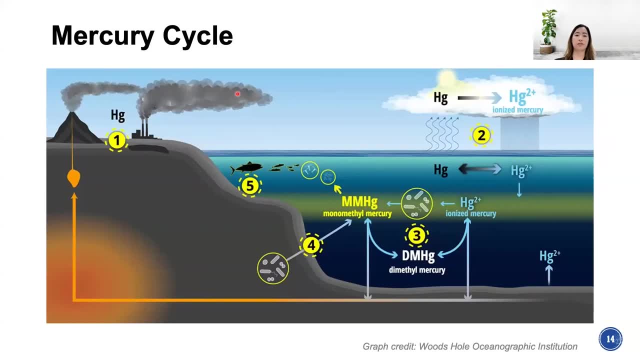 So once they become mercury two plus, they could deposit to the land, to the ocean. Then this is another graph that you know. I mentioned that they come from you know, far away. Then they come, you know, to the atmosphere. 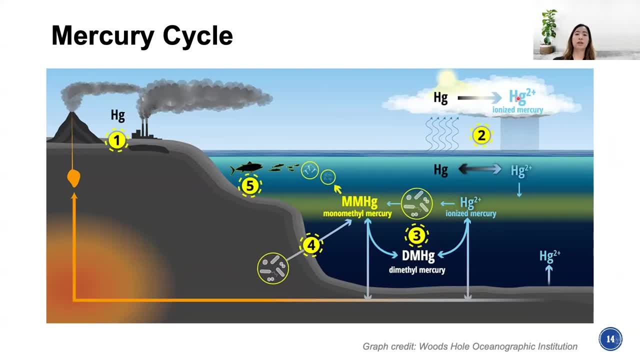 some of them being oxidized to mercury two plus The only inorganic form, you know inorganic form. then they dropped to the ocean. Then this is the time that in some like relatively low oxygen zone in the water it's a favored geochemical condition for bacteria. 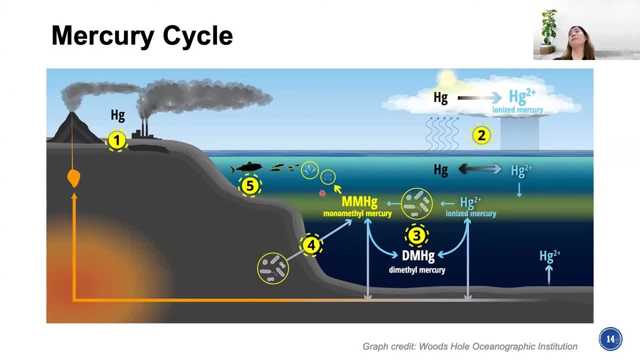 to transform the inorganic mercury to the methylmercury. That's a toxic form. That's also the form that are really easy to be taken up by phytoplankton, then biomagnify along the food chain. So when we talk about biomagnify or about cumulate, 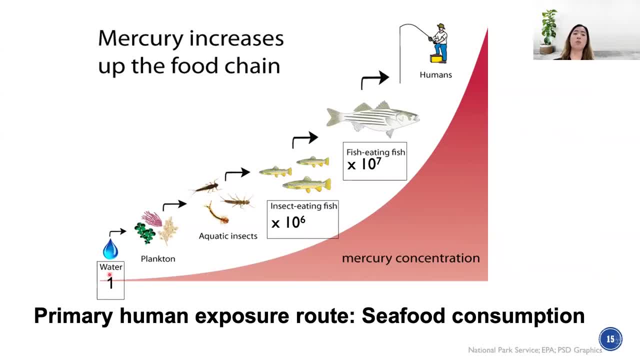 it's really, you know, when we compare the concentration in the water with all the species you know along the food chain. So basically the predators. So methylmercury has really strong biomagnification potential, which means if you compare you know predatory fish. 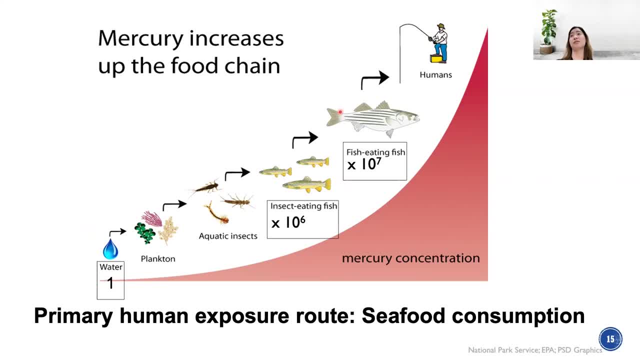 they can have 10 million to a hundred million times higher concentration than the methylmercury. The methylmercury in the water, the methylmercury in the water actually are very difficult to detect, but in the fish no problem. You know, it's really easy to detect. 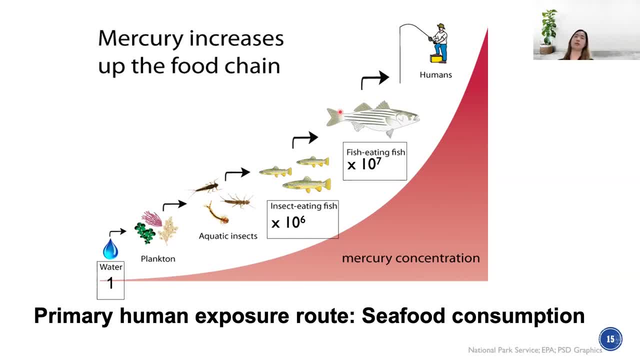 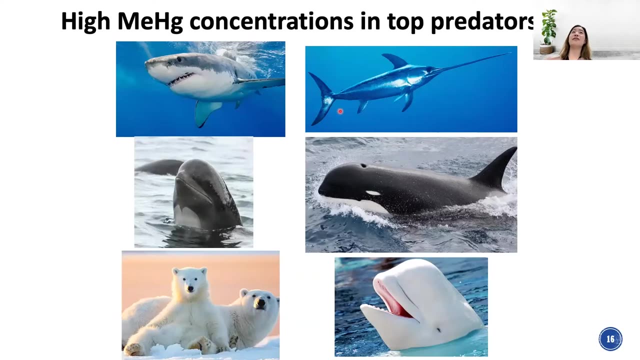 So that's also one of the reasons that you barely hear anyone you know get poisoned by the mercury poisoning due to drinking water, but lots of time we worry about the seafood consumption. So in general, that the larger the fish is, the life. 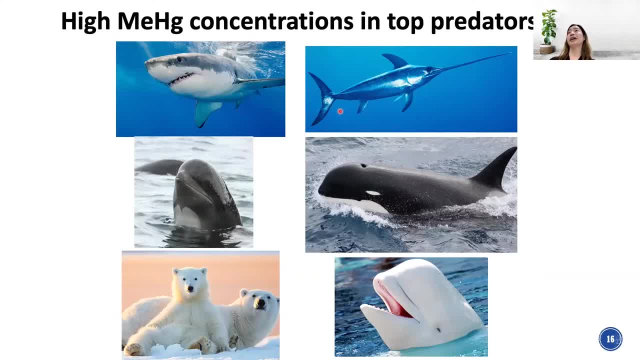 the longer time they can live and the higher trophic they are, the fish or marine mammals have higher concentration. And then remember I already said that mercury is a global pollutant. It could deposit to really far away. So that's why in relatively like pristine. 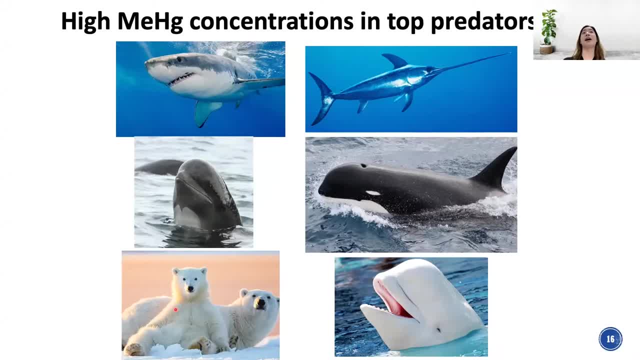 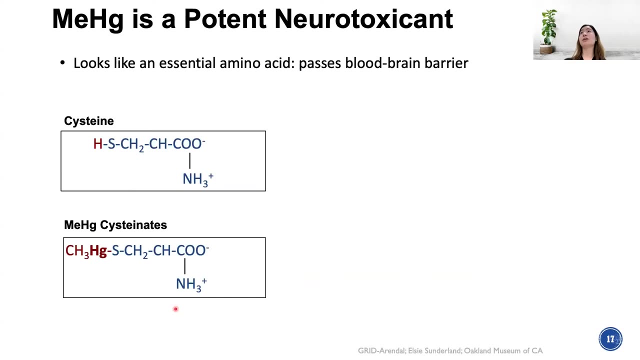 we think pristine environment like Arctic, you find a really high concentration of mercury in their biota, Yeah, So actually one of the highest probably is in Arctic animals, Yeah, So why do we really care about methylmercury? Well, we already talked about it's very toxic. 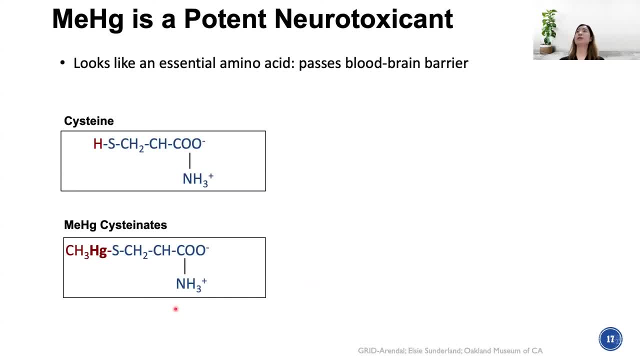 and specifically it's very potent neurotoxicant. So normally biological system have ability to kind of prevent xenobiotic thing to come in right, Or like they can barely come across the membrane because our membrane would consider: this is not part of our body, don't come in. 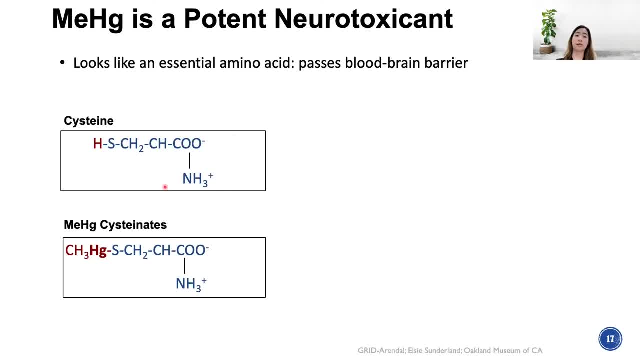 But methylmercury can bind this, you know, bind this amino acid, this essential amino acid that our body need, cause cysteine. They can bind them and mimic, look like you know they are cysteine, So they, our body, actually can distinguish them. 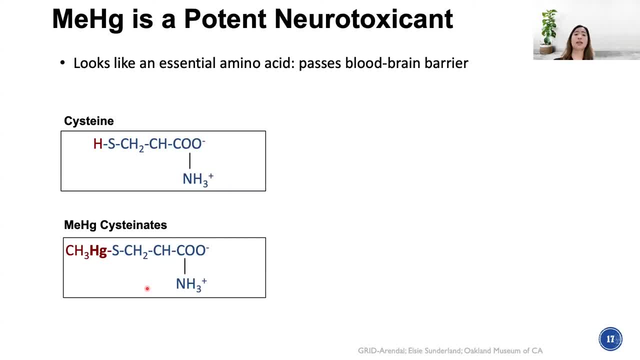 from the amino, essential amino acid And in fact the methylmercury, are very good about crossing. basically, we think, the most like a defensible barrier in our body, which is, you know, the center and the blood-brain barrier. So the central nervous system is the main target. 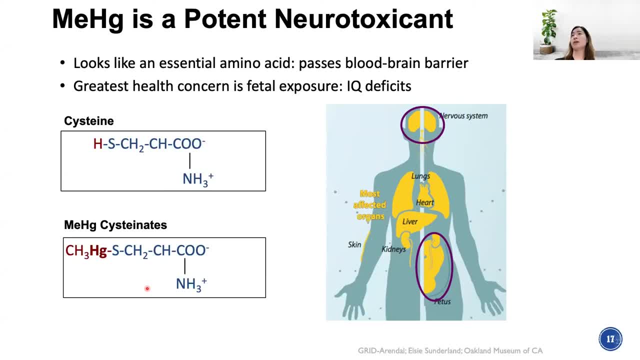 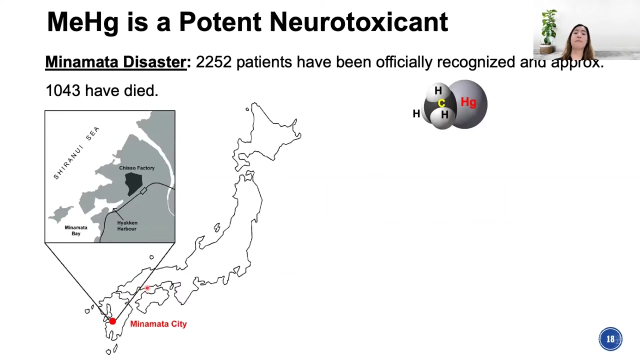 of methylmercury And, as you can imagine, the children and the fetus they are having, this developing stage of central nervous system, So they are particularly vulnerable to this kind of exposure. So we learn methylmercury is poison From a very kind of dramatic environmental disaster. 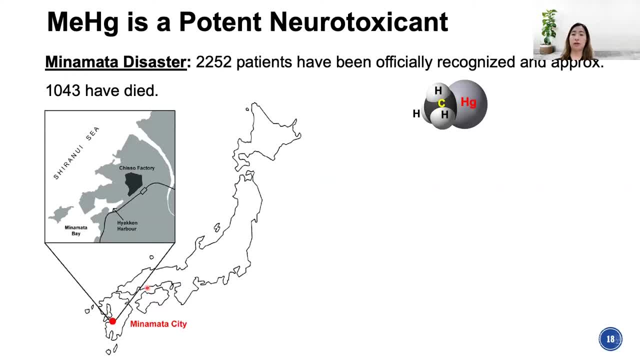 This is called a Minamata disaster, So we got to know this around like 1950s and 1960s. The story is in the in Japan. there's a coastal town called Minamata City, So there is a factory- a chisel factory- there. 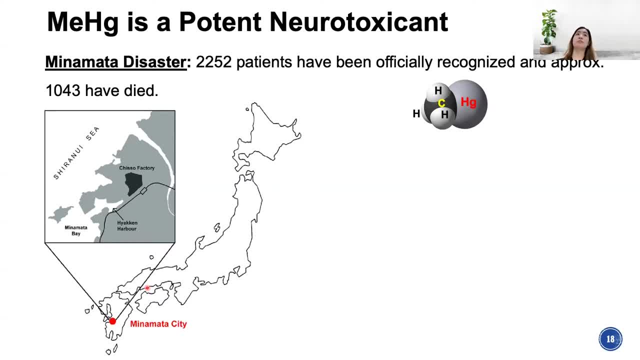 They release a large amount of mercury sulfate into the water. so via their wastewater release And even though this is an inorganic form of mercury that quickly methylated to methylmercury, make this. the bay water and also the seafood in that area has really high concentration of methylmercury. 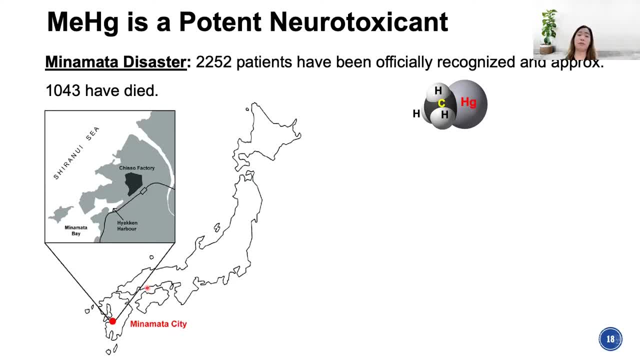 And you know people in Japan, I guess in general, and let alone people on the coastline, they eat lots of seafood And also the cats there eat lots of seafood And they both go basically crazy. So around like 1960s, lots of people. 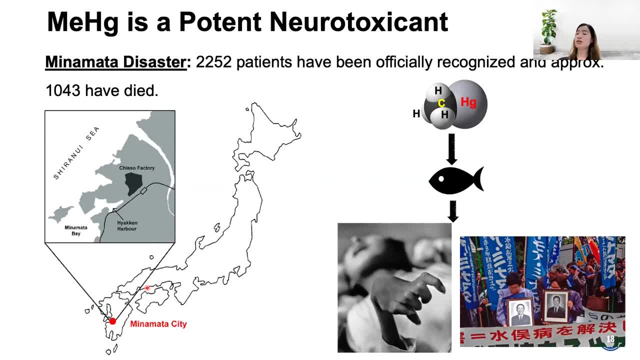 like they lost their vision, hearing and speech, and then relatively severe cases that people have crippling hand and the feet and the coma. So actually you know, more than 2000 patients have been officially recognized and approximately more than a thousand people. 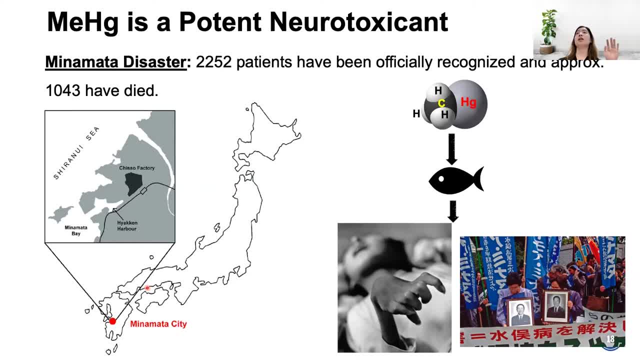 have died of this disease And the lawsuit between the people there and the factory and maybe government is still ongoing, And even you know, after so many years. and one thing I want to mention is because methylmercury can pass the placenta. 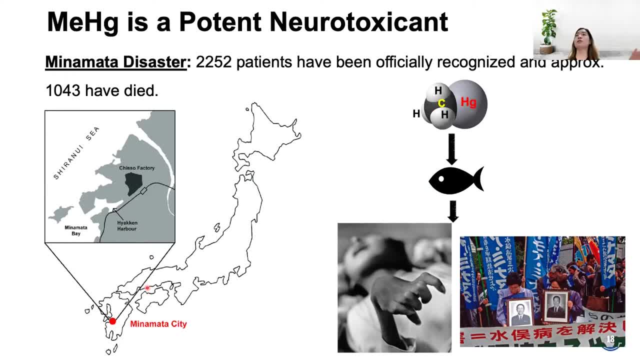 so they can pass from generation to generation right. So I think that's also why this whole impact is still lasting for so many years, Although we wouldn't have such a kind of a dramatic case anymore, because most of the country has a regulation about their wastewater. 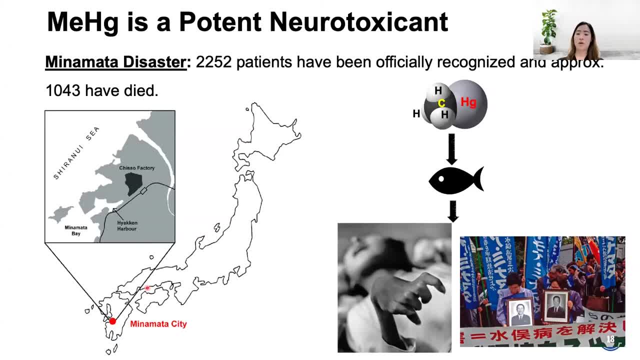 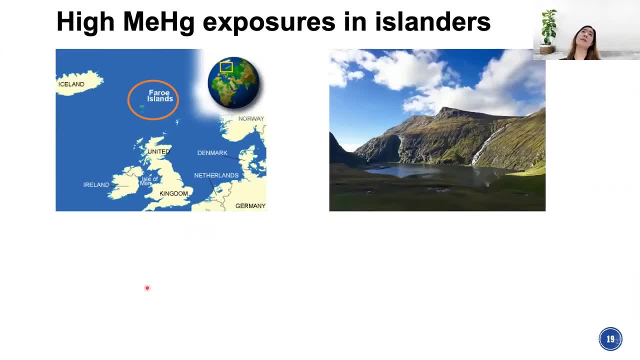 You can't directly release so much into the ocean directly, There are still a problem. I guess many, many people in the world still have very high methylmercury exposures. So that's my PhD work that I did kind of focus on Faroe Islands, which is a beautiful island. 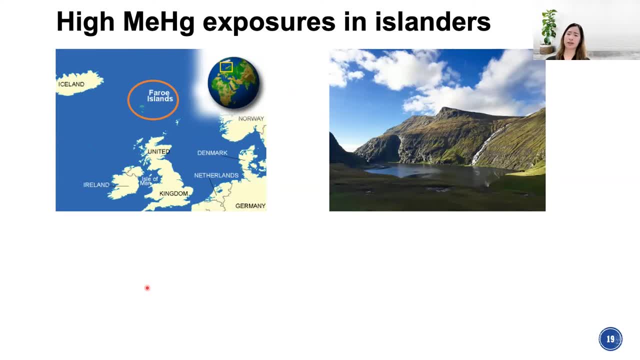 which in kind of between UK and Iceland. it's actually a self-governing archipelagos under the sovereignty of Denmark. So they are- because of weather- they're super windy for most of the time of the year- that they actually can't like really grow. 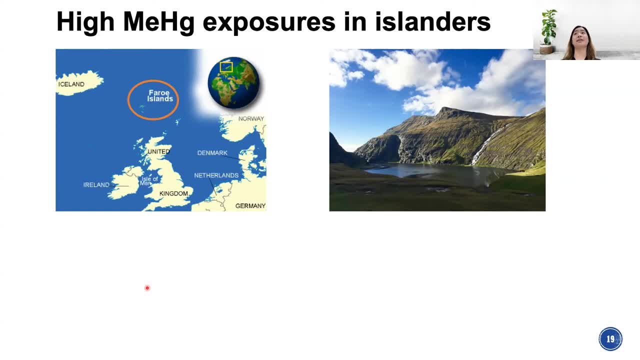 that much vegetables They also don't have like a local livestock you know like. so there's the researcher coming from them, the islands that their kid the first time when they saw a squirrel. they call it dog because they don't have squirrel. 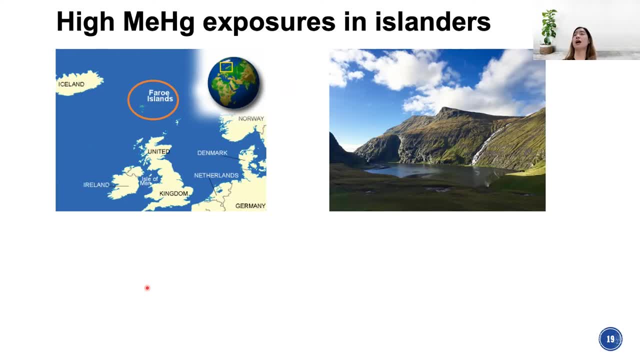 they don't have rabbit and they start cultivating. you know the cows and lamb sheep there, but that's not the normal thing they have there. They just they eat seafood. that's what they do And that's lots of Islanders have as well. 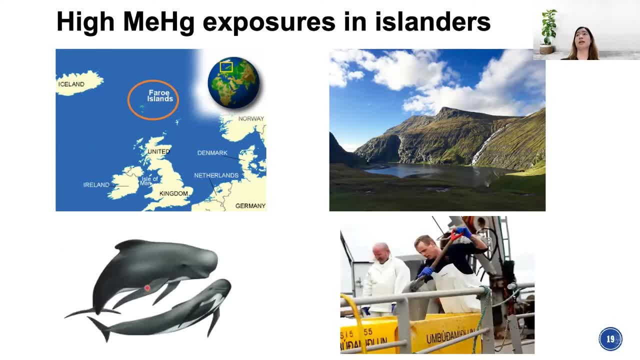 And traditionally and culturally they eat pilowail meat and liver. So they do have annual hunt of that. And so there are a group of scientists- you know of the group of scientists or some kind of some sort of what do they call them? 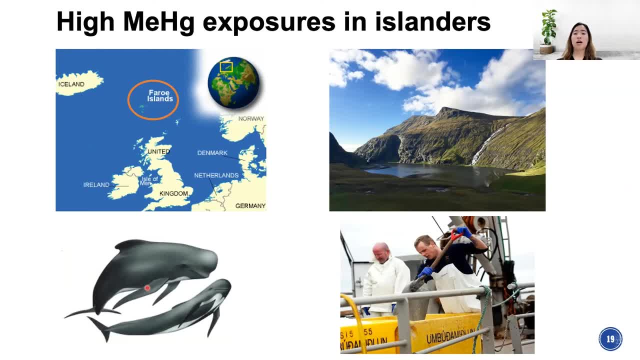 a group of scientists that study mesometry, um, and we think that the population may be at risk because pilot whale, as a top predator in that ecosystem, has very high concentration of mesometry and the people there, you know, been eating them for a while, so they basically the 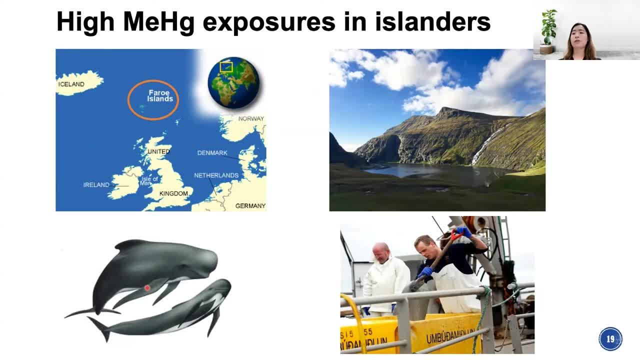 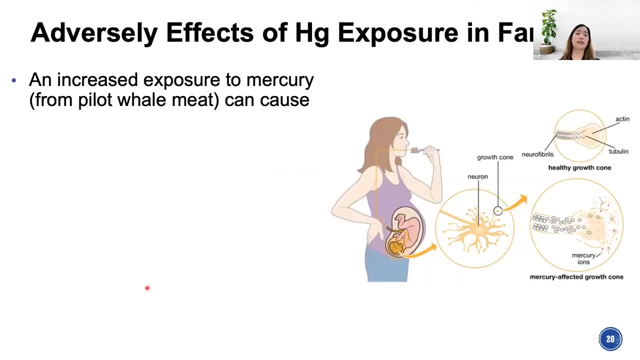 epidemiologists set up a cohort and follow the women and the baby and over years, and also set up a lots of tests, you know, to understand the potential neurological effects over time. so what they found is that an increased exposure of mercury from pilot whale meat and liver consumption. 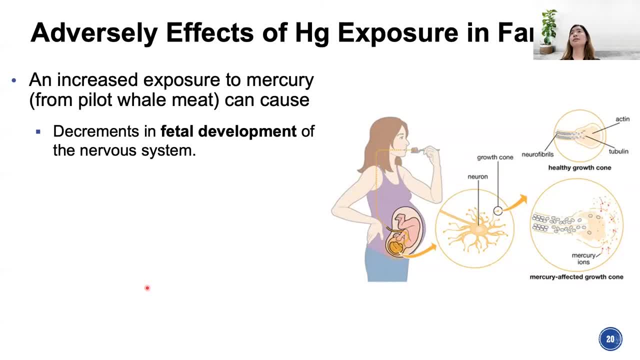 can cause the decrease in fetal development of their nervous system. it also will cause a cognitive deficit in young children with the prenatal exposure to mesometry, so in other words, their iq will be lower than their peers. and also for adults, there could cause risk of increased risk of cardiovascular disease. so this is actually 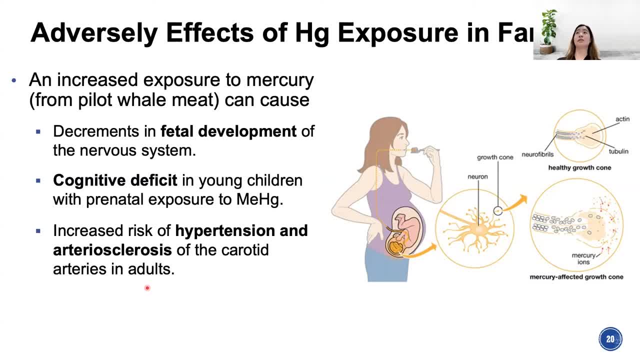 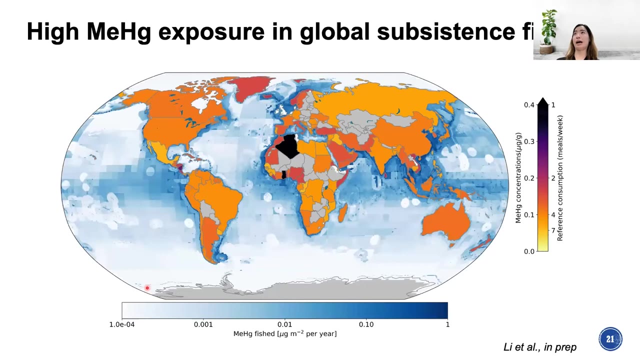 really important and solid evidence and that's one of the very important evidence base that our us epa actually kind of based on when they developed the reference dose of methamphetamine exposure for us population. yeah, so just kind of plugging a little bit that not only um, you know the. 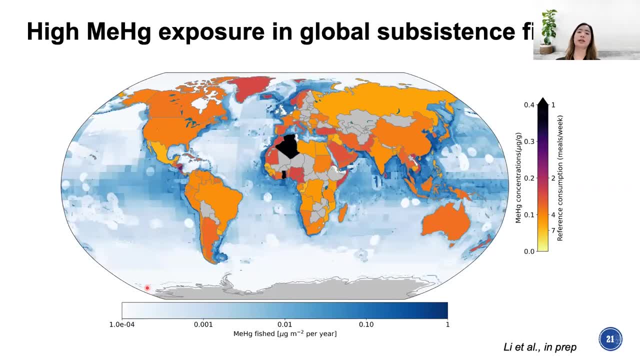 farah islanders. um, so my current work actually take a look at the global subsystems fishing populations. by definition, they fish for food and we found that most of these populations are at risk if we use us population, us reference dose, that set established by epa. so this is you know. 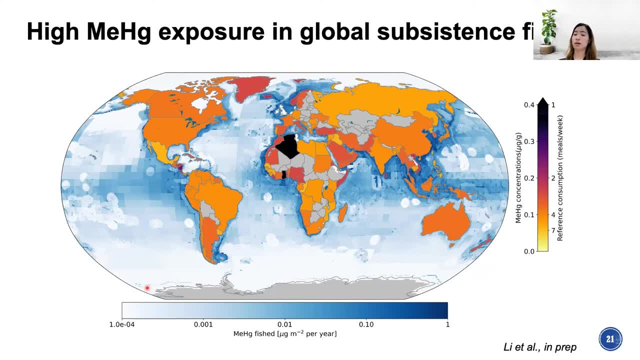 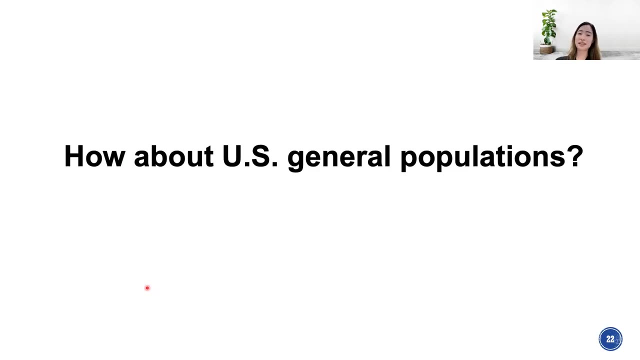 kind of really show. based on the current level of methamphetamine in the ocean, it still poses direct threats to many populations in the world. So how about US general population? I think that's what most people are kind of interested in. So we started a project that we basically 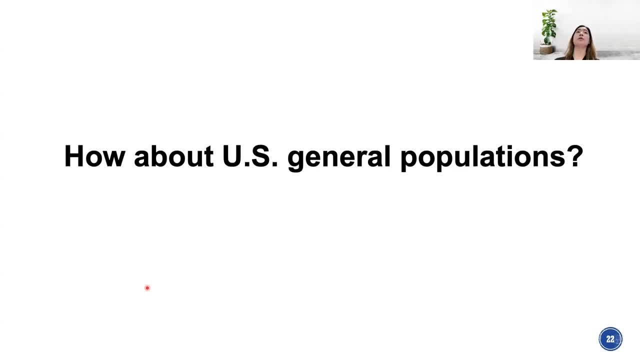 take a look at in general like a seafood commercial market in the United States, and we take into account the import, export and domestic lending. So the leftover is the ones that we really consume by US population. What we found is, first of all: 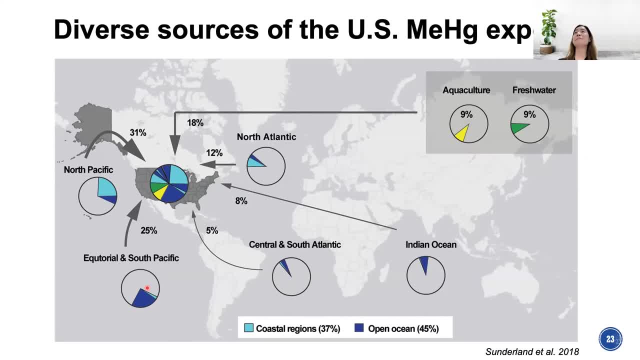 this country really gets seafood from everywhere, all the ocean basins. So basically you get methamphetamine from all the ocean basins, Again highlighting it's a global problem And in addition, that for the US. you know, if we break down to different seafood category. 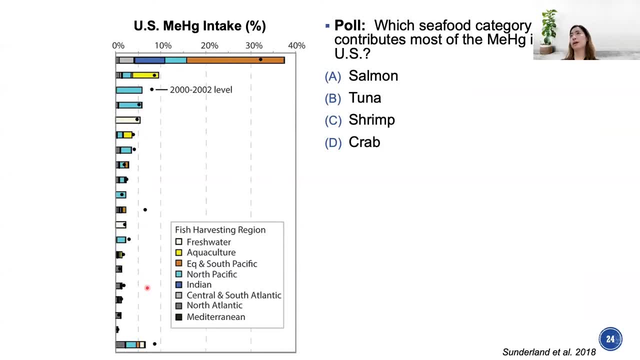 which I made a bar chart here. so different color of the bar are just different fish harvesting region And the height of the part means you know how much percent of that seafood, how much percent of methamphetamine total intake is from that specific species. So I guess we have a poll that we can open on the Zoom. 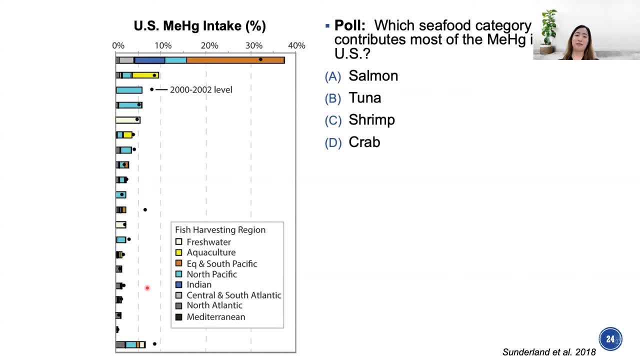 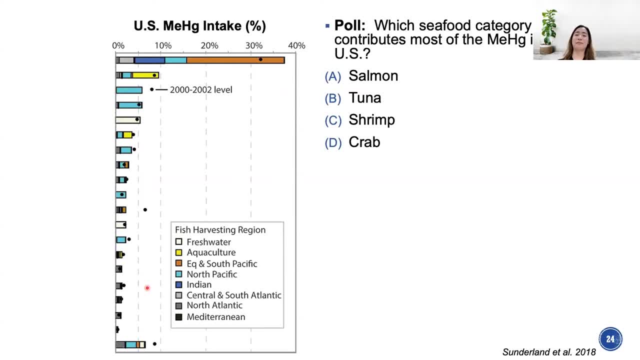 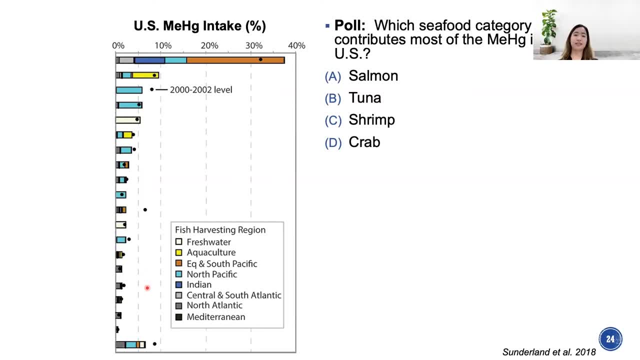 I think A, A okay, Sorry, 3. B- okay. So we have three B and one A, and I don't know how many. maybe we'll give a little bit like five more seconds for the 3.. 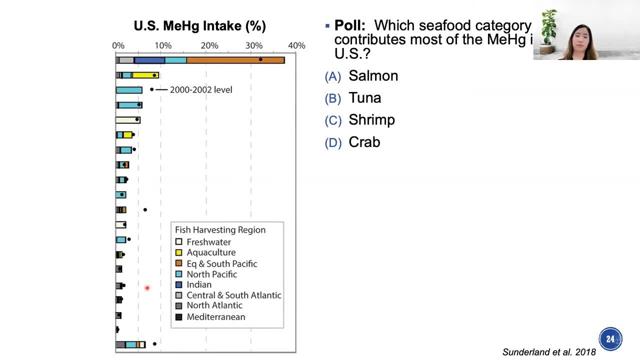 So, yeah, welcome to have other answers if you have, and then we can In a minute. 70% of people answered: Oh, okay, Yeah, so we have more bees here. so how about you? Yeah, mostly tuna, 70% between them, and secondly, salmon. 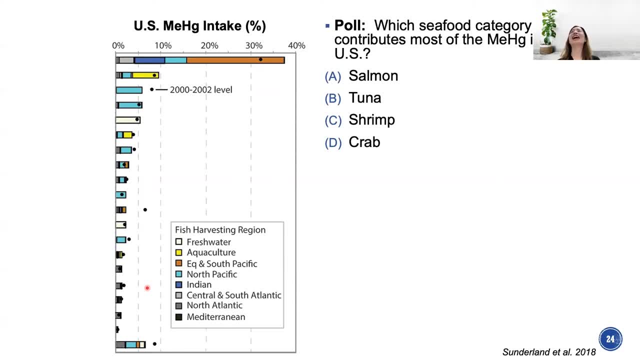 Okay, so well, it's quite matched right. So I guess people are knowing like tuna, because I mean they're both big fish, right. But the one thing I want to mention is so the answer. I guess let me go to the answer first. 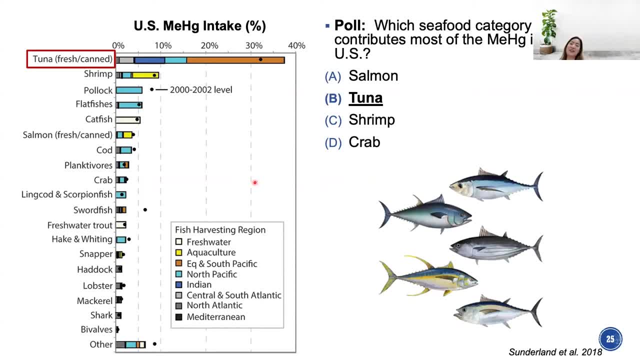 The answer is tuna. So the reason so we eat them a lot. first of all, it is true, but the main reason is tuna has a much higher concentration of methamphetamine than the salmon. So remember, they're both top predators. 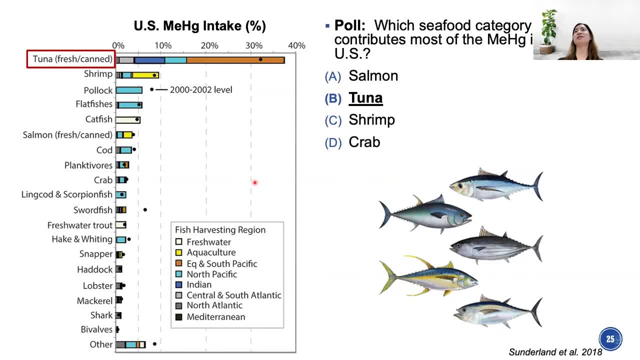 but salmon usually only live maybe three to five years. Tuna could live 30 years easily, right, And also I guess there's also where they live that make a difference as well. But in general salmon doesn't have high mesomercury concentration. 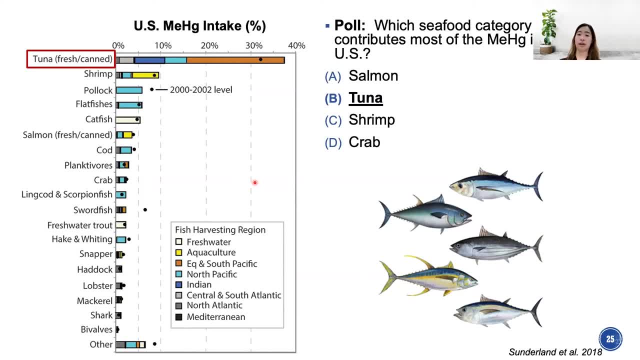 It's actually relatively a healthy seafood choice. But I guess most of people I think good job, And so I guess we get into species level And I mean for this country you can tell most of the mesomercury is actually contributed by basically one big group. 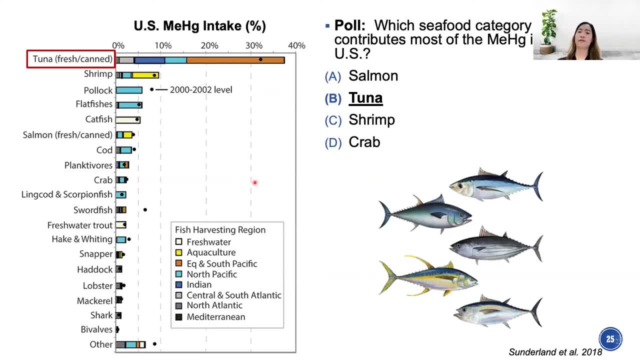 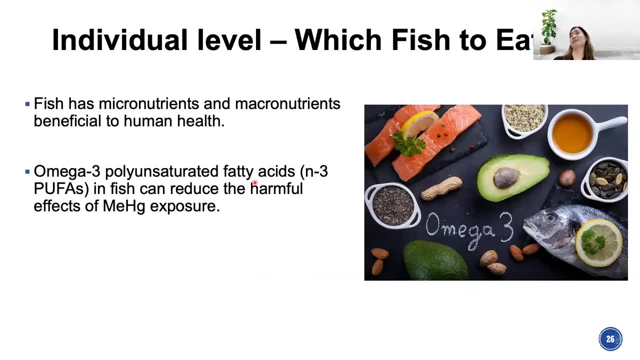 And lots of time when I go to a conference and people would ask me this question: what should fish to eat? Because mesomercury basically is in all kinds of seafoods. I don't want the message would be like: don't eat seafood. 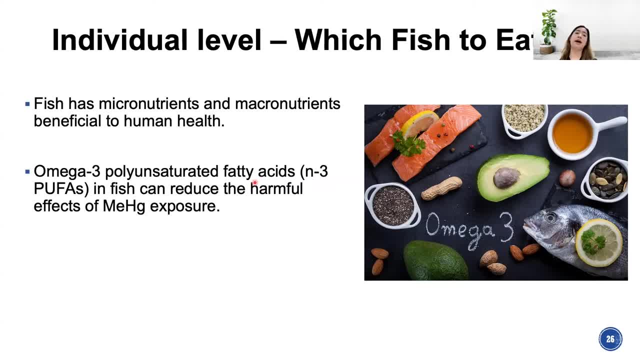 Fish has- yes, fish has chemicals inside. They also have- yes, they have- seafood have lots of important micro and macronutrients that are beneficial to human health And more important that some micronutrients, for example, omega-3 polyunsaturated fatty acids. 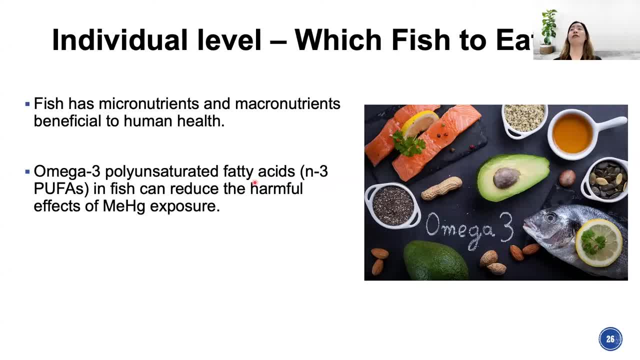 in fish that actually can reduce the harmful effects of methamphetamine exposure. So they actually have a counter. you know effects And the most important I think everyone should remember is fish that is high in methamphetamine are not necessarily high in omega-3 fatty acids. So you can be wise about what you want, what you eat. right, You can try to. 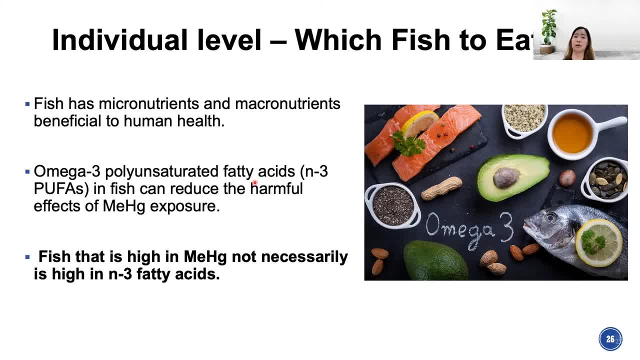 maximize your benefit and minimize your methamphetamine exposure, And at individual level, because we can actually change. you know the seawater methamphetamine concentration overnight or the seafood methamphetamine concentration. But what we can do is we can be wise about what you eat, I think. 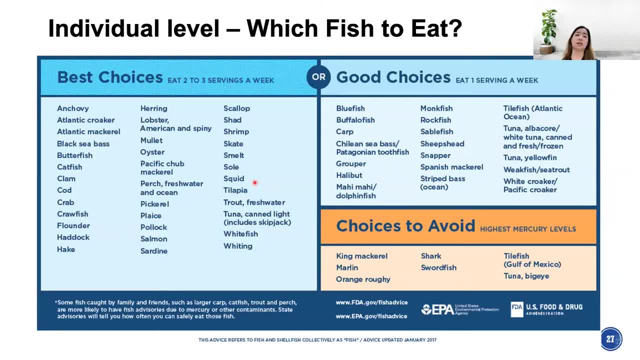 So this is the FDA, and EPA actually developed a kind of fish consumption advisory. So if you Google, you know FDA fish consumption advisory that's published in 2017, they actually tell you the best choice, the choice and the bad choice, Like I mean, they will tell you: avoid big eye. 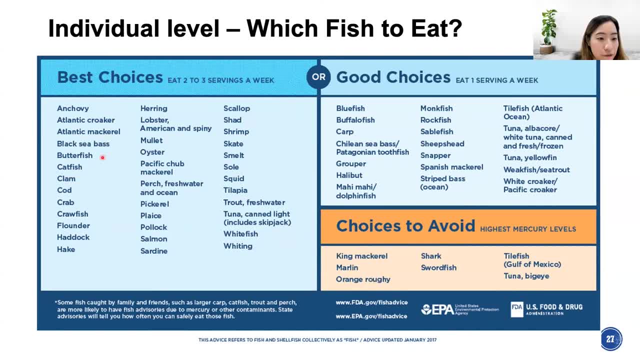 tuna And salmon actually is, I think, one of the best choice, if I remember. And also, yeah, yeah, Because salmon is fatty and it has usually has lots of omega-3 fatty acids. Yeah, So that's something I think we do, like you know, individual level, But what we can do at the global level. 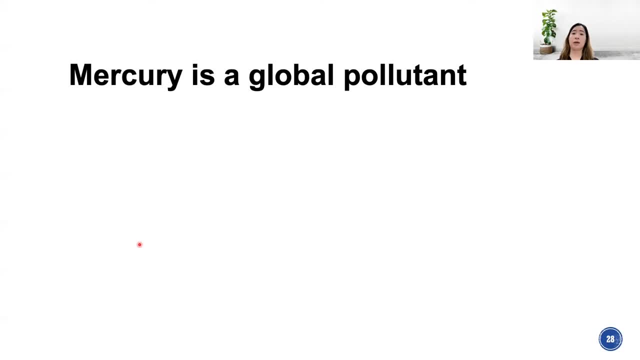 right, because it's a global pollutants, especially for United States. we get fish from everywhere, right, That's the fish. In order to reduce the human exposure, we really have to have global regulation right, And I want to end this talk by saying thank you so much for joining us. 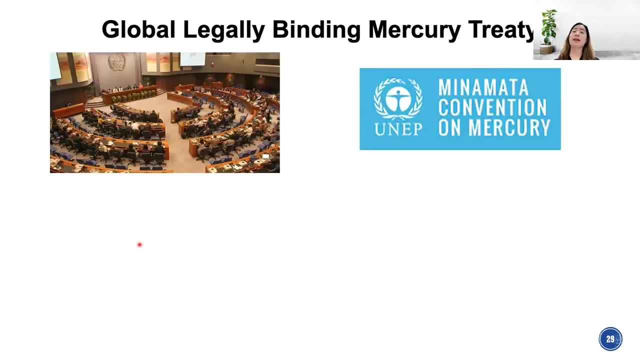 I want to end this part with a kind of positive note that there is a global, legally binding mercury treaty, which is the first time that there's a treaty, a global treaty, as just for one element, It never, ever happened. It has been, you know, scientists and the politician and the non-NGO. 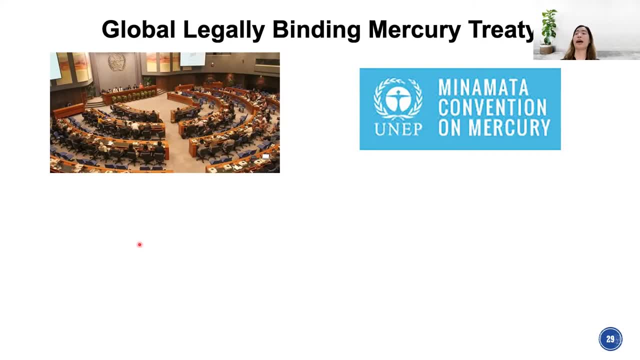 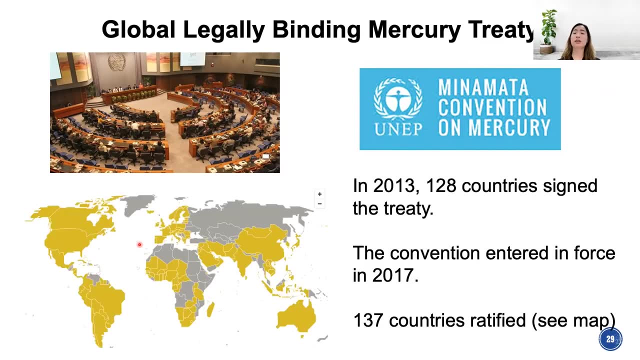 all these people have been working for decades to get that happen, And what this mean is in in 2020.. In 2013,, there are more than 100 countries that signed the treaty, so they agreed to reduce or minimize mercury emissions in their country to you know atmosphere or to environment. 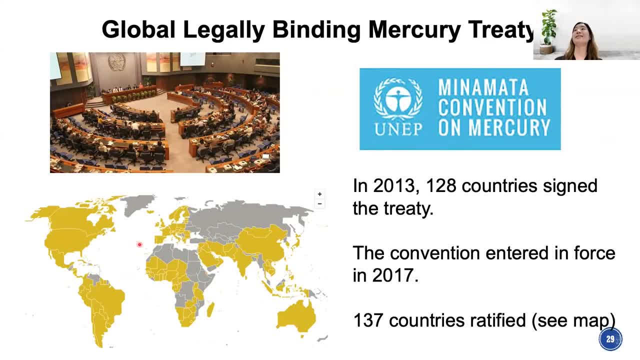 And this convention entered into force in 2017, and I checked it yesterday- that 137 countries ratified. so this is a map here that the country that ratified. So the ratification means that they have already have their own national regulation in place and this reduction of mercury emission is happening, which is very promising, and hopefully in the near future, there will be a long list of good choices of seafood right for us. 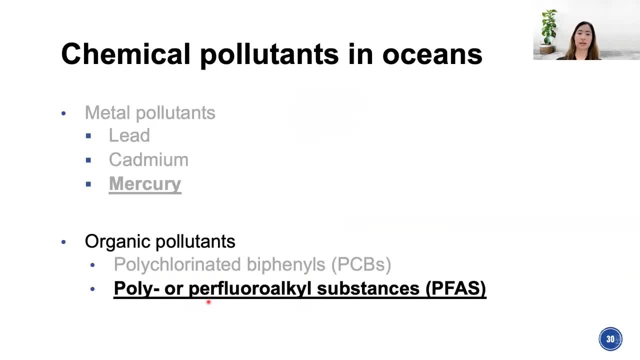 So for the rest of the tonight, and I want to talk about another type of contaminants which is organic, So organic pollutants. in short, it's a PFAS. It is very different from mercury because it's not naturally occurring. it's totally man-made. 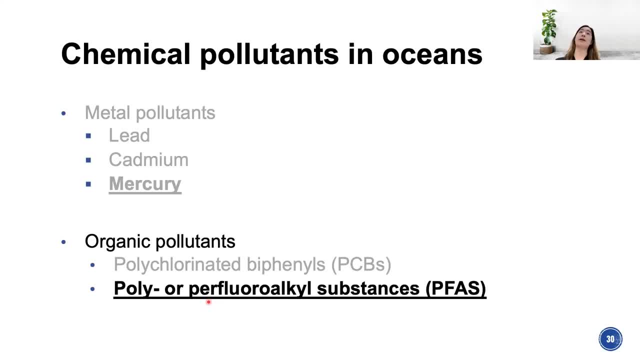 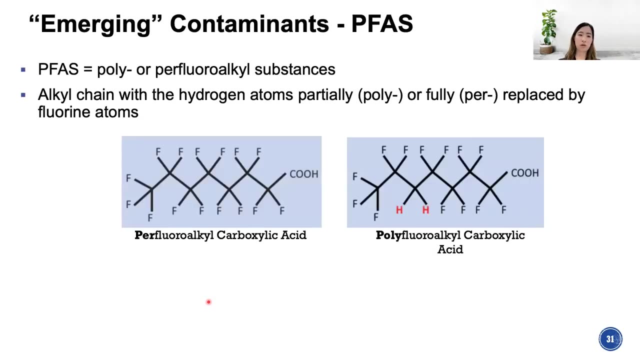 And second, we know relatively little about that, and mercury will have been studied for a while. This one we studied since 2000,. so it's quite relevant and the scientific evidence is just coming out quite rapidly. So just in case you, 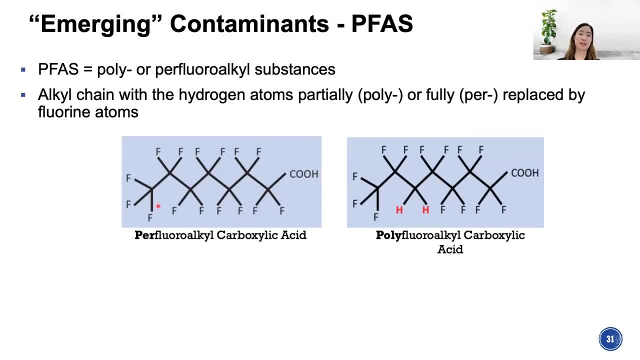 like molecules and like these photos, that the, the PFAS, is a type of a very larger group of chemicals that they all have, like this carbon backbone, and they connect it with fluorine atom. So so this is problematic because the carbon fluorine bond is probably the strongest bond in organic chemistry. 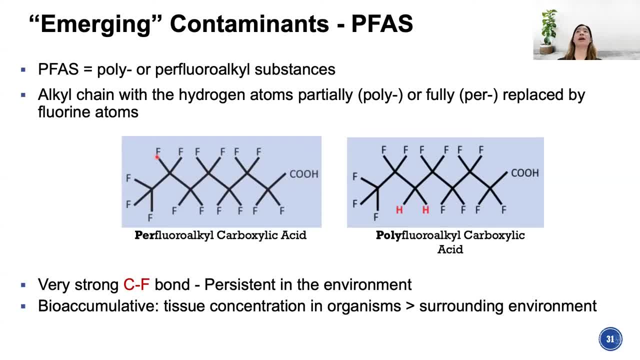 It's very, very hard to break them down. We can't find microbes or something that in natural ecosystem that can break them down. So make them super persistent in the environment And some of them are bioaccumulative, which means you will find the tissue concentration in the organism higher than the surrounding environment. 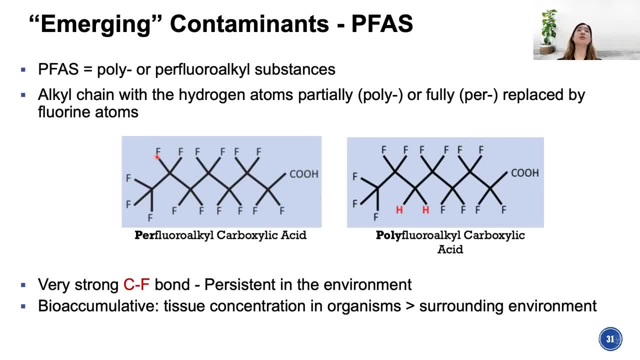 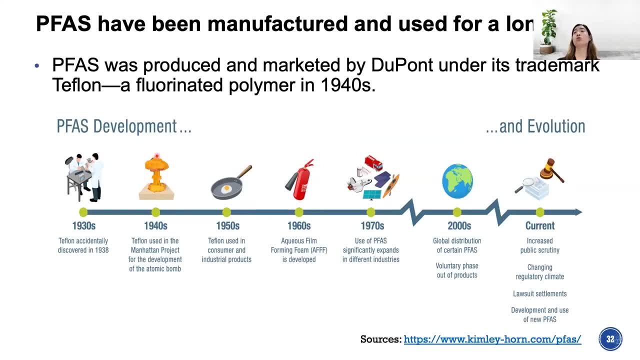 We actually call it emergent because the signs are emergent. We have been using it again for a really long time, and it's the. In 1940s, DuPont was the first one that produced and marketed under their trademark that Teflon. 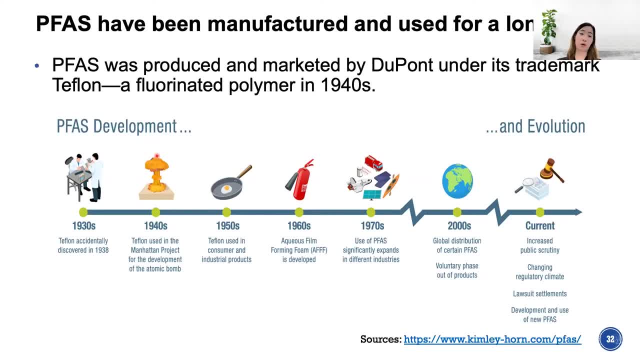 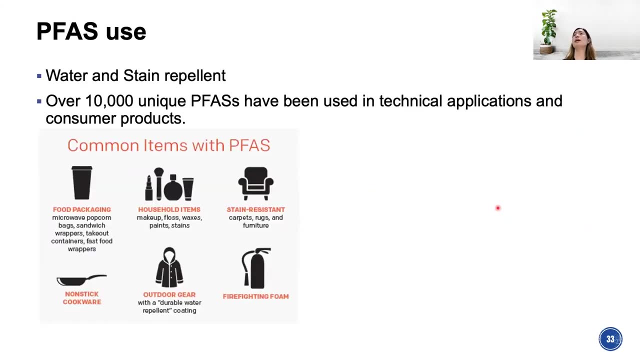 So it's a you know it's. we have been using them for a while and so since 1940s there are lots of other products that have been using this, this whole group of chemicals, And the reason we use them is it's really good surfactant, so it's water and stain repellent. 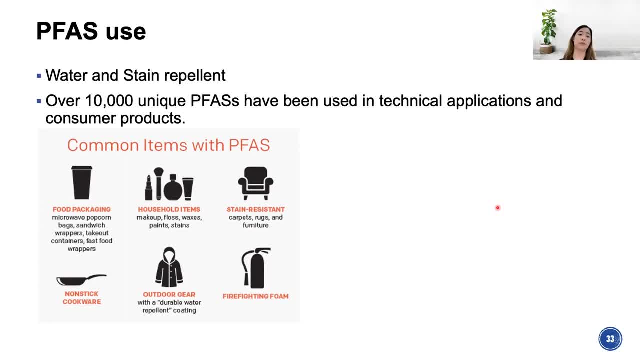 So it is really useful And I mean I'm glad that you know we found that property And now over 10,000 unique PFAS have been used in technical application and consumer products And then you can imagine right stain and water repellent- really good for food packaging. You don't want the oil or water you know penetrate when you get something from Starbucks or something. 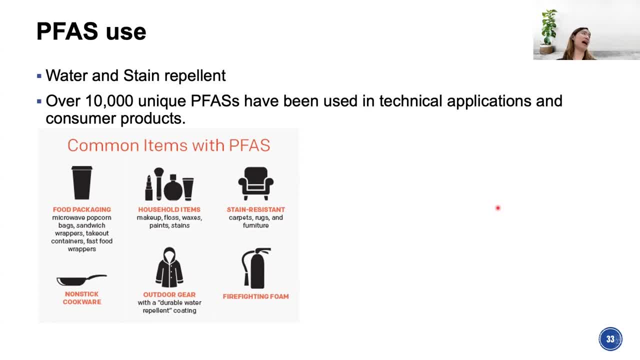 And household items- makeup, you know, eyeliners, lipstick- lots of them show that they have PFAS inside dental floss, stain resistant furniture, carpets. They also have PFAS and non-stick cookware that have been known for a while. So if lots of time we go to store now they will say PFOA free or PFAS free, that's because before they used that. 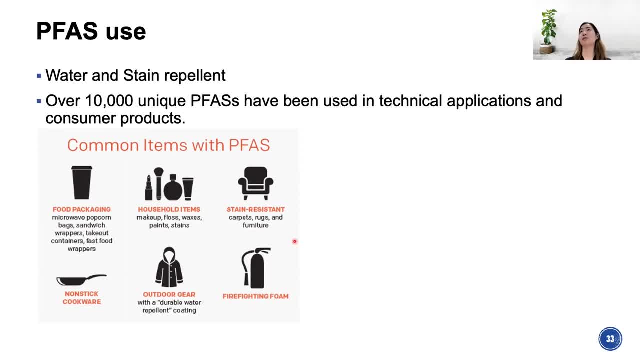 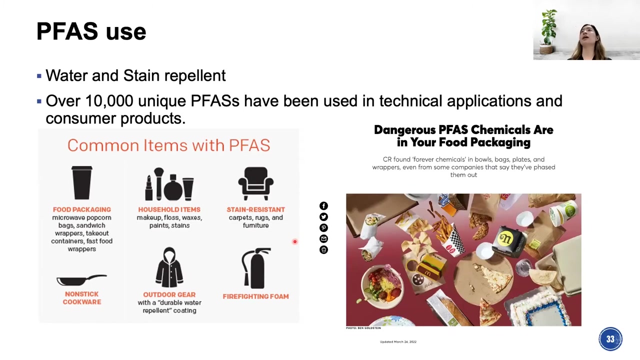 So another huge contributor is firefighting practice, because PFAS widely exists And so the airport or military bases are usually the point sources for PFAS. So just a kind of recent study that published in late March this year that they found PFAS widely exists in most of the food packaging in the kind of fast food chain that we, you know, see all the time. 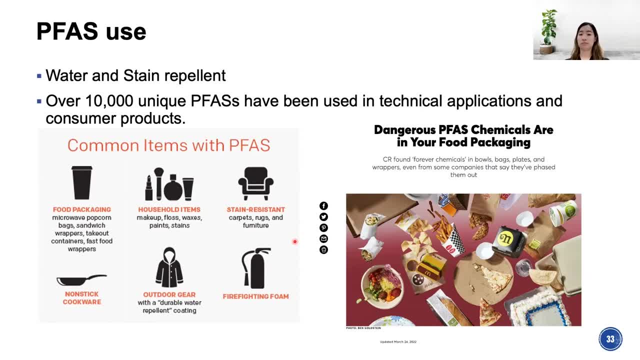 Some even claim they don't use it, And so you know there's a lot of evidence that you know it's being detected. So just give you a little bit sense that you know this is kind of everywhere almost. 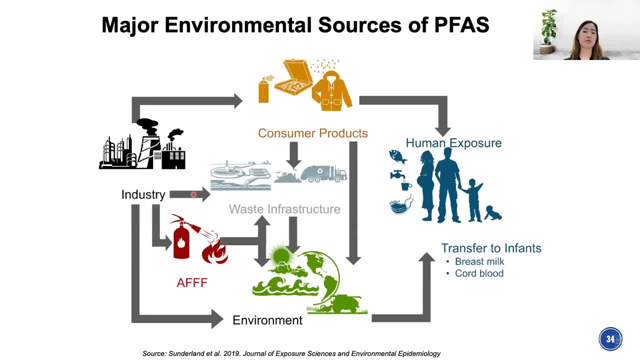 And so from consumer products or industry. eventually, PFAS come to the waste infrastructure. right, And the waste infrastructure again. these compounds are so hard to break down- The waste infrastructure not designed to break them down- And they become like a source that they collect in them, they enriching them, then they released to the environment. 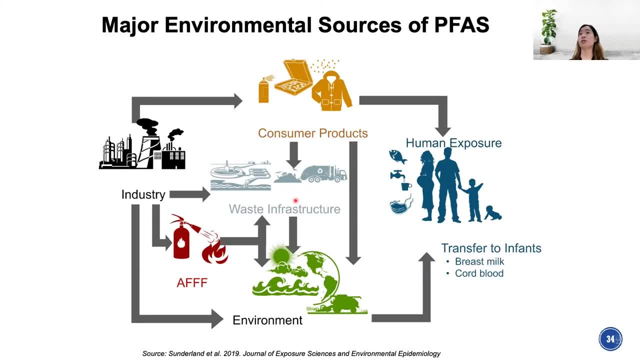 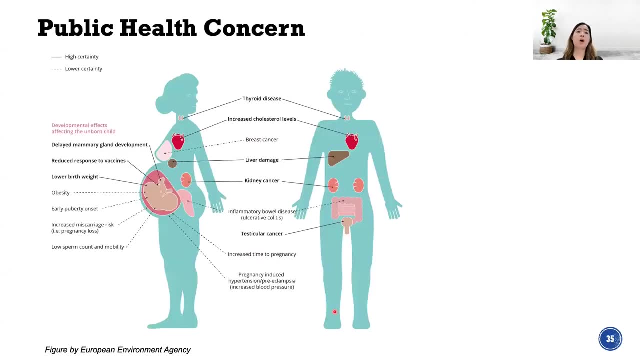 And so waste water treatment plants or landfills are usually also a point sources for PFAS, And eventually these PFAS you can imagine transported via the surface water or groundwater then to the coastal area in the ocean. So why do we care about PFAS? 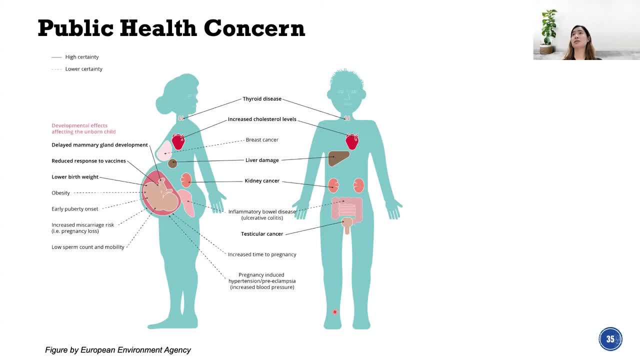 Lots of studies show that with high certainty that PFAS is toxic in different ways. It's associated with many kinds of cancer, It reduces the birth weight and it can be a very strong immunosuppressant. means like your vaccine wouldn't work And because the PFOA and PFAS are two types of PFAS, that 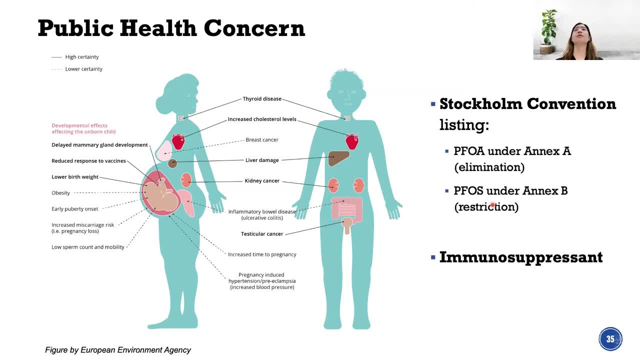 have been well studied and because of the health effects that they have been listed on the Stockholm Convention, which is a global convention for kind of phasing out the really toxic persistent organic pollutants. But again, PFAS has 10,000, no more than 10,000 compounds in this and the 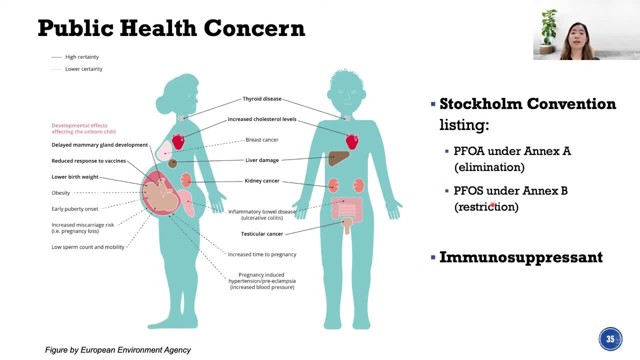 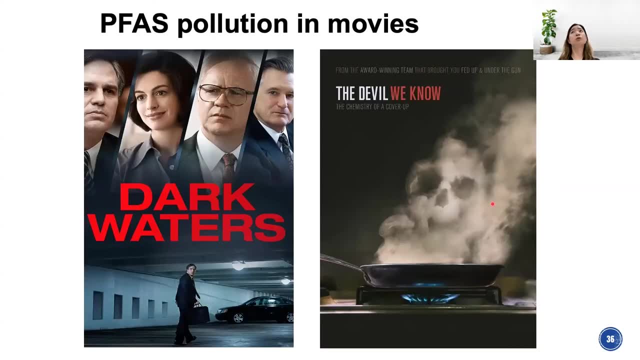 majority of them has not been regulated yet. But just in case you know, if you want to know more history about you know PFAS application, what kind of health effects? you can go to the Stockholm Convention website and you can find a list of all the health effects. There are two. 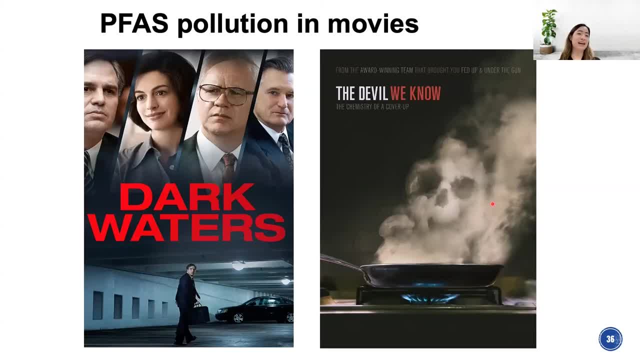 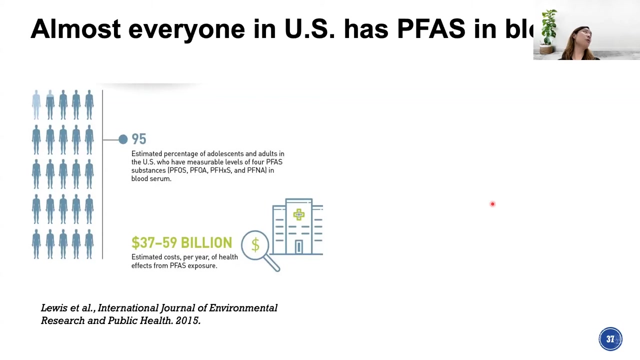 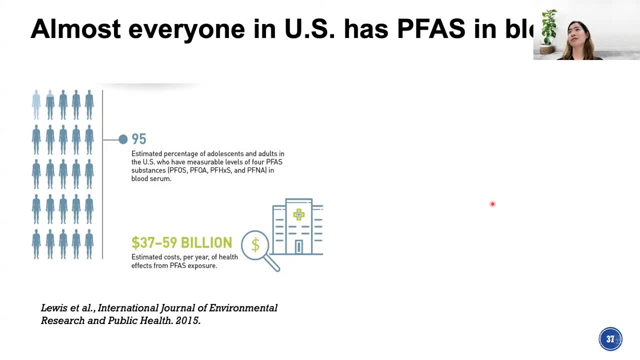 talk about it a little bit later. But I'm going to talk about it a little bit later. But actually- and this is a horrible study- that they look at a population we call NHANES. so it's a National Health and Nutrition Examination Survey. So the CDC actually survey people that represent the US. 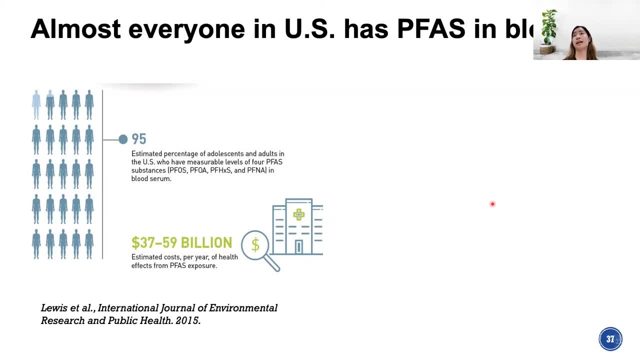 general population every couple years for their nutritional status, health status, And they found 95% of that population, which represent the US general population, has PFAS detectable in their blood. Again, these are data that did not come from the US general population, but from the US. 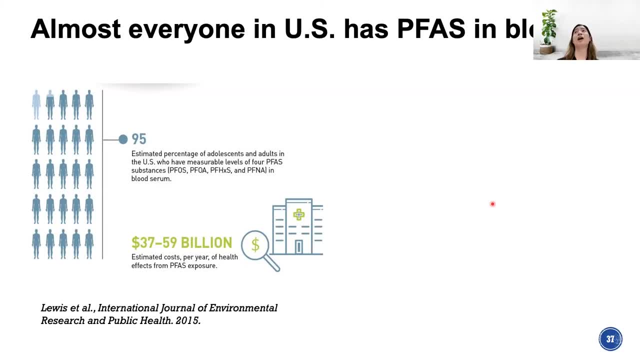 generation And so this is a study that they looked at. a population we call NHANES- so it's a national- are man-made things that we don't really need any in our blood, And I saw new studies that are coming out as even higher percentage. So essentially everyone here that have PFAS, you know, have 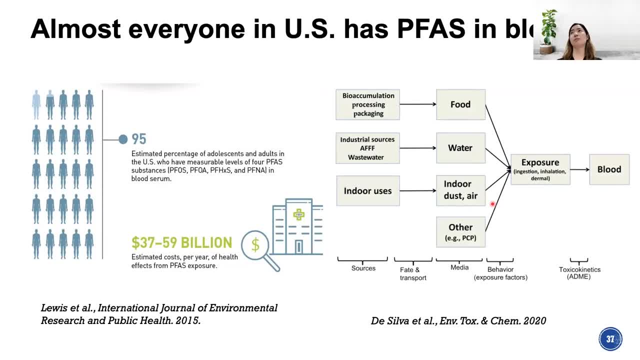 exposed to PFAS And in terms of where you really get them, really varies depending on where you live. So if you live in a place that drinking water has been included by PFAS, then drinking water is probably the main source, But if you're not living in drinking water contaminated area, 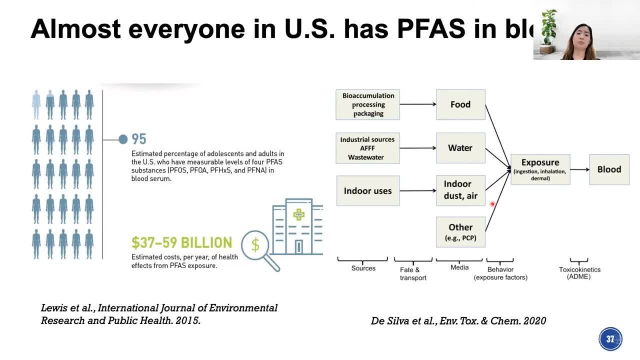 then not predominant pathway is probably food That could be from, you know, by accumulation in the seafood. That could also be, you know, these packaging that you know eventually the PFAS doesn't get onto the food. So right now we don't really have a national regulation. They. 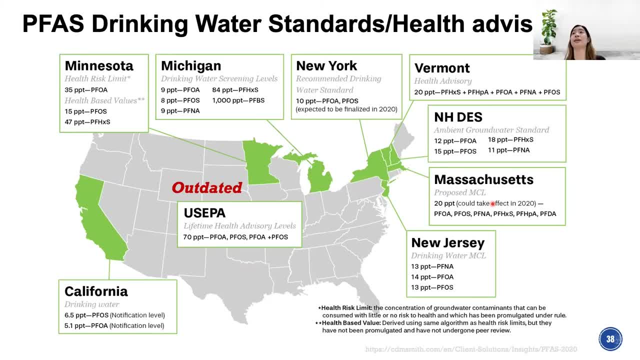 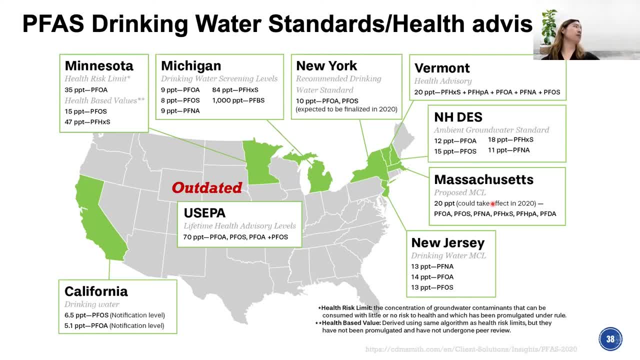 want to show you why you know this is still important. So until last month we're still using US EPA's 70 ppt, so nanogram per liter for PFAS and PFOA maximum level as kind of a national 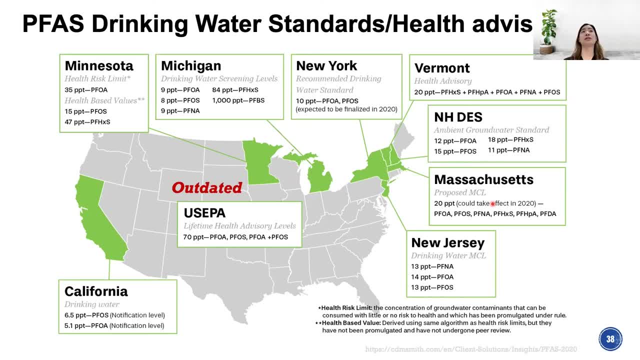 level And we all know from epidemiological studies that this is too high For protecting human health. That's why all these states that have lower concentration or stricter standards for their drinking water or surface water- And I think Delaware is coming up and very similar to what New Jersey has- is around 10 ppt, But last month US EPA actually issued 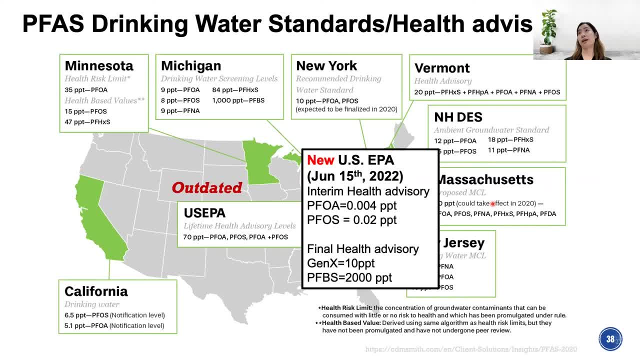 a new interim health advisory and the final health advisory for another two type of PFAS. But if you compare PFOA and PFAS, previously they were 70 ppt, Right now they are orders of magnitude lower. They are so much lower that most of the waters in the country probably cannot. 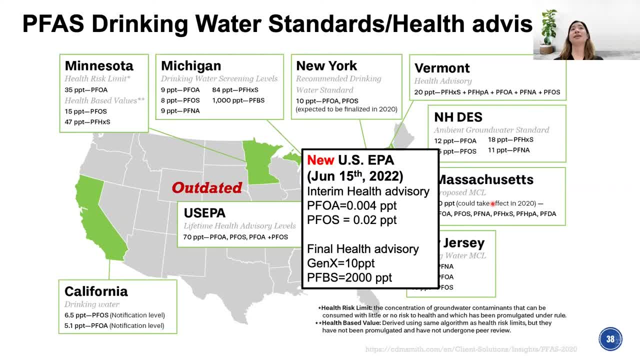 achieve that. But I just want to tell you why they get this. So they got this as they consider a safe level because that is from an immune toxicity study in children, And they back calculate how much the maximum level of PFOA Drinking water should be for protecting the most vulnerable population. 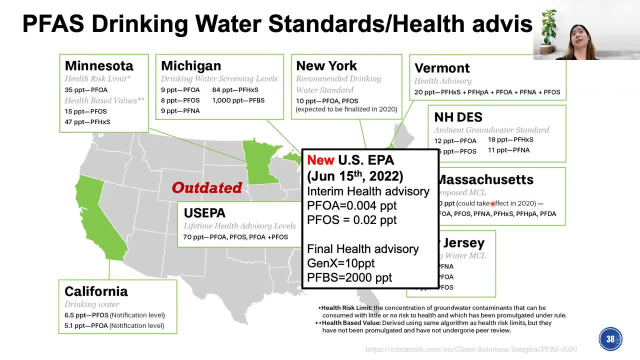 So as from a public health perspective, that's totally valid, Right? But that also shows, because I mean 70 ppt maybe most of the place in the country can accomplish, But the people you know less than one ppt most of the place can't like probably. I mean, I test my lab water. 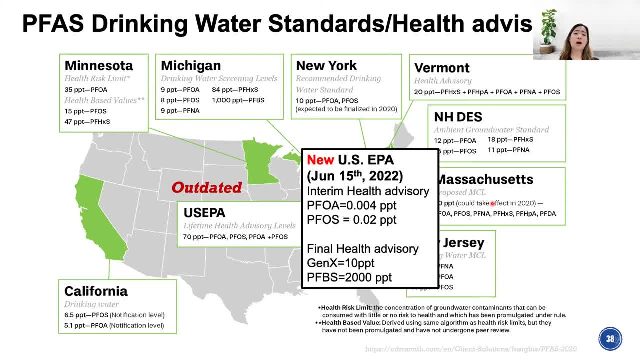 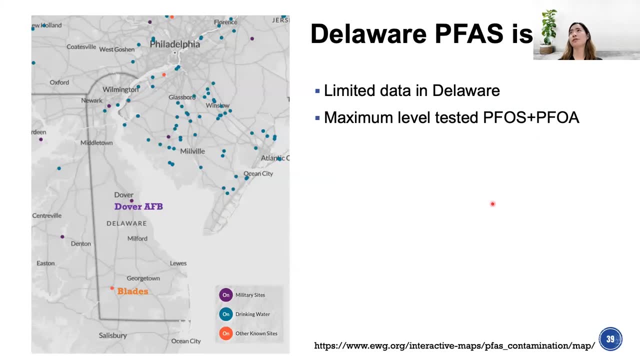 That's not you know. it's exceeding that level. So that's also long for you know. if you think about it as like, you get a goodО. this is a map that you can go online. it's ewgorg. They have an interactive map that you know. 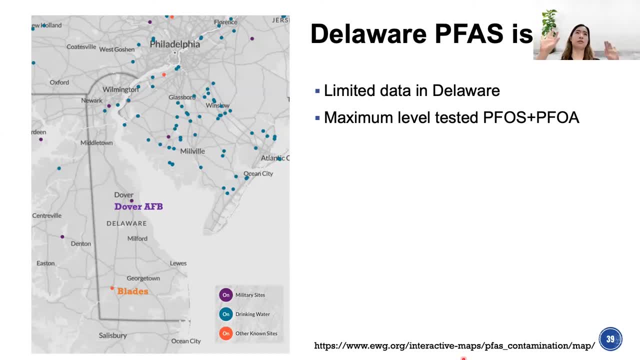 anywhere they sampled or they collect data from, like a place that sampled for drinking water or groundwater and every data point on the map just shows you like you know they sample there. then there's data. so it doesn't mean it's necessarily being polluted, but you can tell. 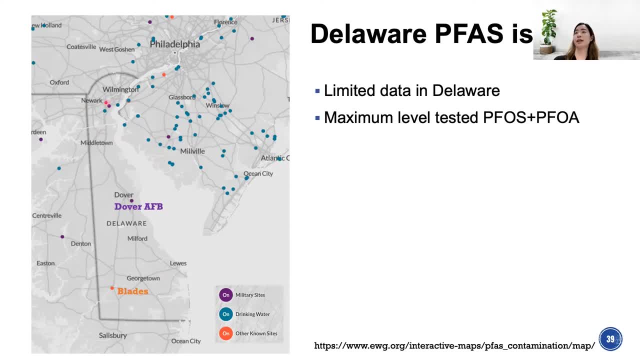 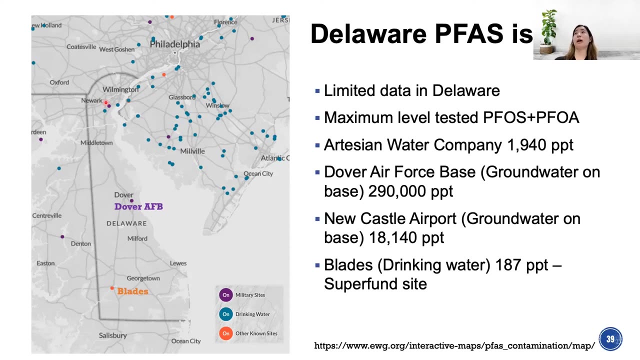 that you know, Delaware is pretty empty and not so many data there. right Like, I believe Danrock is working on that, but we're still kind of slightly behind with, like you know, compared with New Jersey and among the ones that sampled are very concerning. so I was saying 70 is too. 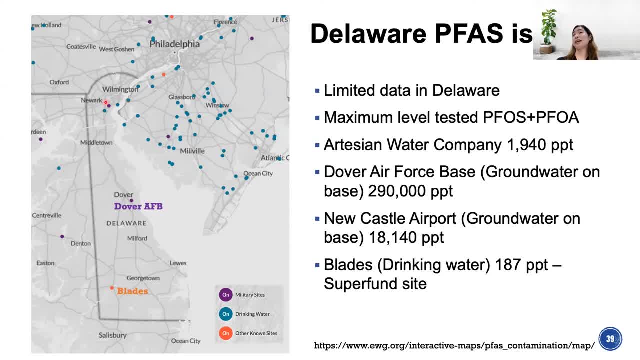 high. These numbers are not. you know something you like to see and I believe the Artisan Water Company that's in Newcastle they have. I've already installed the filters because that's not something you know they want to supply. 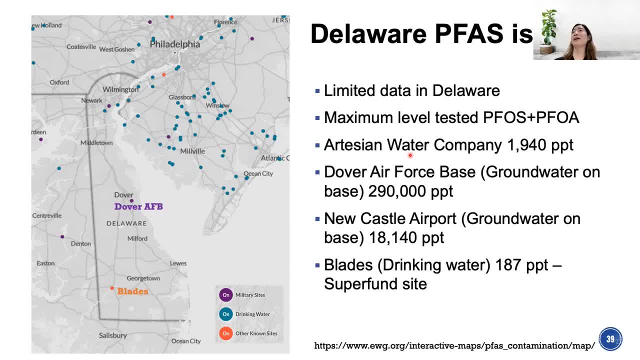 people, but I mean they have been supplying water for a while and the Blades, which is not far from here, their water is polluted by, I think it's a local industry. so that's higher than the old EPA health advisory. therefore they become a superfund site that EPA and, I think, collaborated. 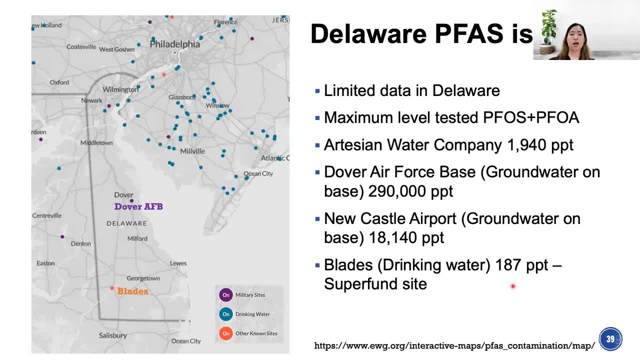 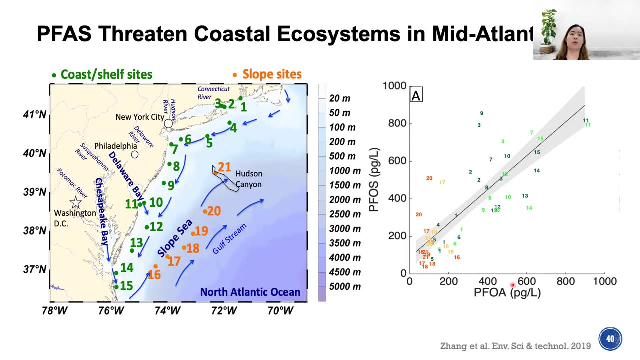 with Danrock are cleaning up now that site. So compared with drinking water, so most of these are drinking water groundwater. there are fewer data actually in the coastline, so this is the one I can find that's relevant to. you know our area, So they sampled seawater inshore, offshore. 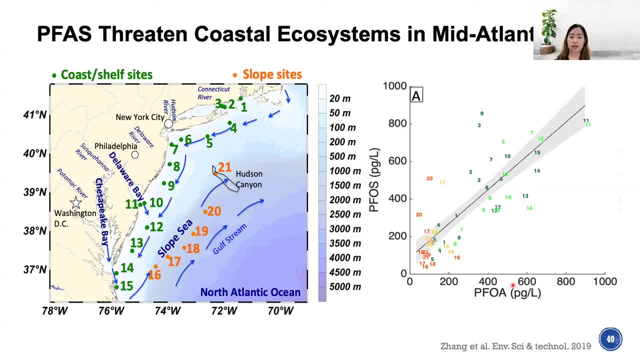 from New England to Mid-Atlantic. then they found that you know where who has the highest right. So it's right, It's right outside of the bay. They didn't sample inside the bay, So right outside the. 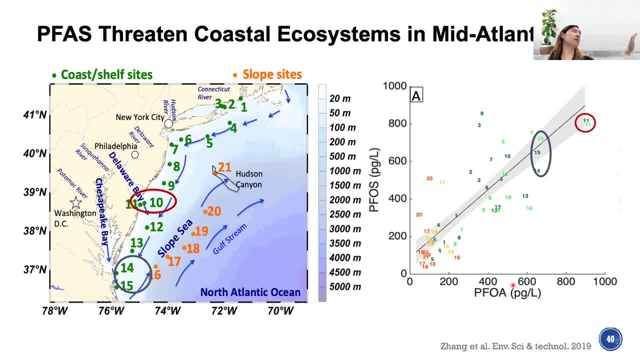 bay of Delaware Bay- that is the highest among you know along this coast and the runner-up has Chesapeake Bay, So kind of highlighting, you know, regionally we probably have big issue of this, but not so many studies actually are like following up, like published, yet 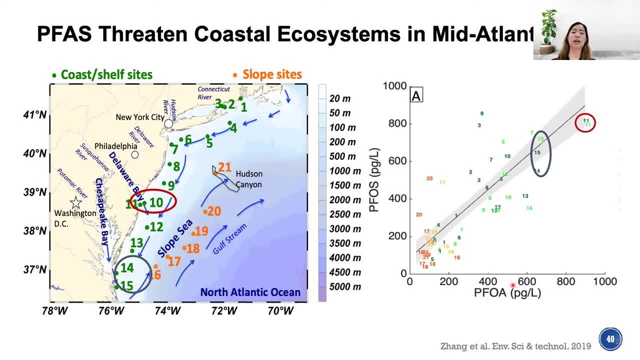 so that's the only thing I can find, And that's also something that really kind of struck me, and when I started a little bit over two years ago at UD, I decided to take a deep look at it, especially. you know what happened in the Delaware Bay, right? So the question: 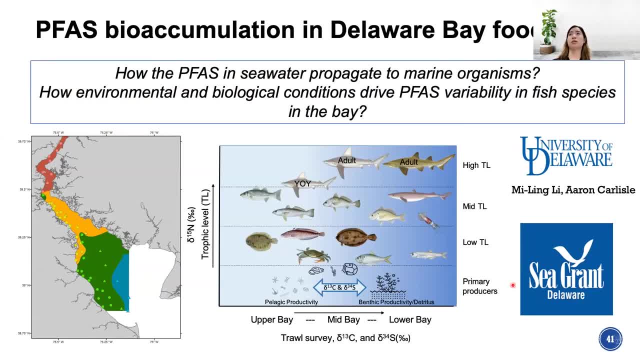 I have is you know how is the you know the distribution of PFAS in the seawater, in the sediment in the bay and how high the concentration in our marine organisms, and how you know are there any species that are particularly vulnerable or in other? 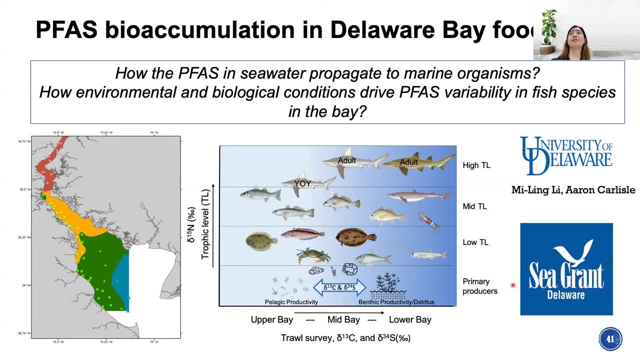 words have much higher concentration than others, because these questions directly relevant to human health and also for animal health, right. So that's something in my mind and we applied for a Sea Grant and that's ongoing research that funded by Delaware Sea Grant. 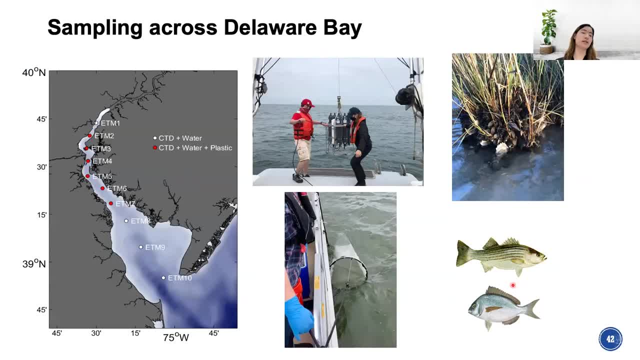 And we have sampled a little bit in the bay and the plan was, you know, going through the whole food chain and you know sample environmental samples and you know the samples and biological samples. So far I don't really have data for you guys, but 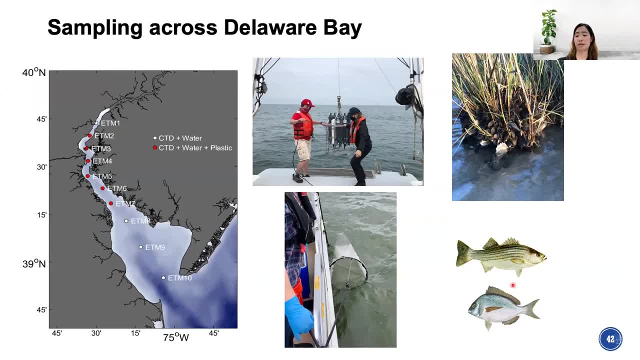 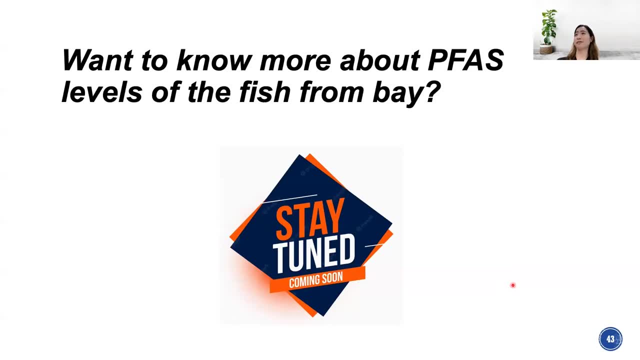 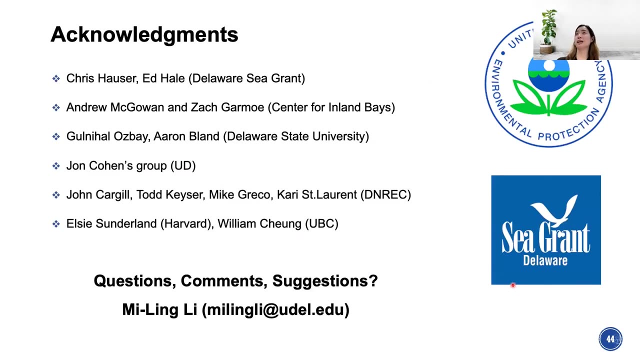 you know, a year from now I should have plenty of them, and so if you're interested to know more about PFAS levels, you know, of the fish from the bay, stay tuned, You know, maybe come back next year around this time. Yeah, so I think that's basically all I have today. 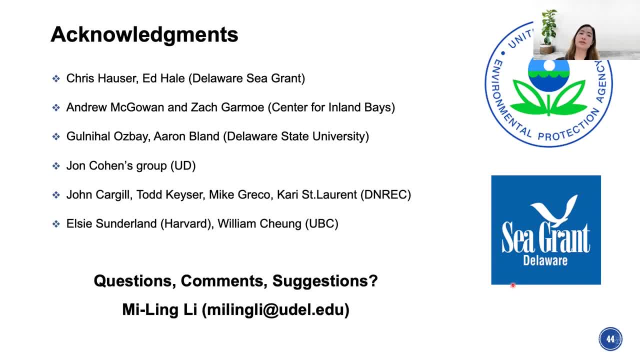 and I do want to acknowledge my collaborators and especially people from Delaware Sea Grant, and, you know, I think that's all I have today. Thank you. A big shoutout to the Sea Grant, Chris Hustlen and Al Hill. I started my career at UD during. 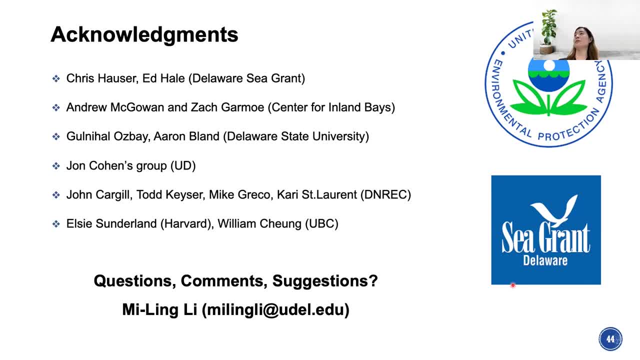 the pandemic without knowing much about the state, knowing much about you know people here. So these two are really directing me to lots of helpful resources in you know Center for England Bay, Delaware State and the DAREC. So I'm not going to say every. 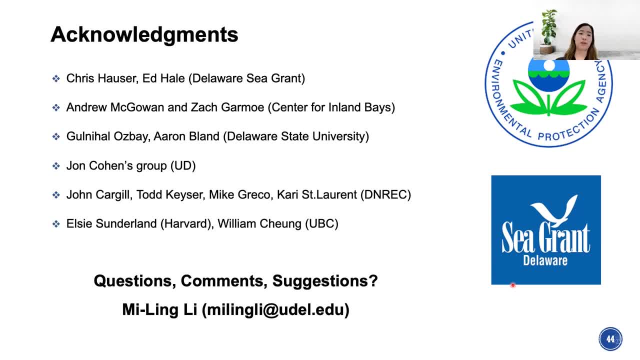 of the names here, but I'm very truly appreciate their help. Also, John Cohen's group at UD. they've been our field trip buddies for a while, so, yeah, special thanks to them as well. The work I presented about mercury is funded by US EPA and I want to thank my collaborators. 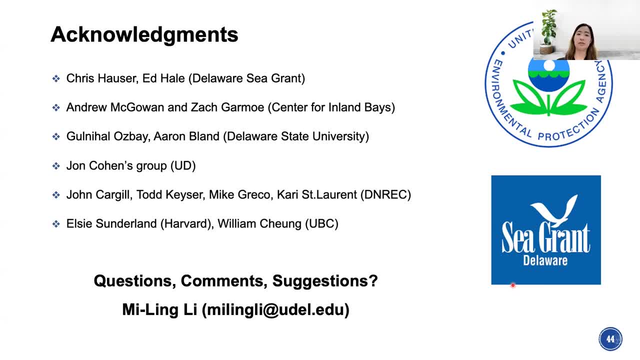 at Harvard and UBC as well. So I think hopefully we're on time and I'm happy to take questions or comments, suggestions. Did anyone measure the mercury levels right down here in our water And or grab the fish or two and measure the mercury that they catch right here? 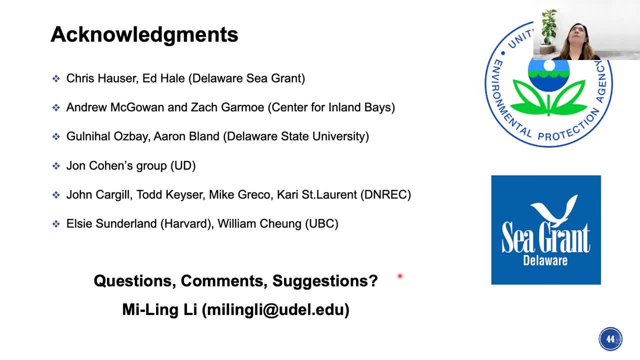 I don't think so. So the question is: anyone measure the mercury from this area? I think there is. if I remember correctly, there's a study in Chesapeake Bay, there's a study in the Long Island Sun, I don't remember. there is a particular study in Delaware Bay, especially about fish. 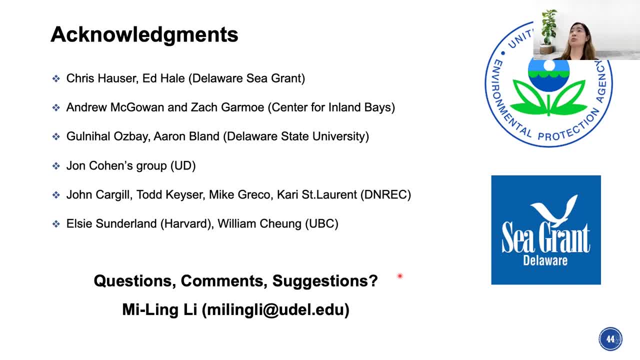 But I believe at least the river fish, like the freshwater fish, is definitely monitored in terms of their mercury level, their PCB level are monitored by DNRC And that's why, for recreational fishers, make sure you check out the state level fish consumption. 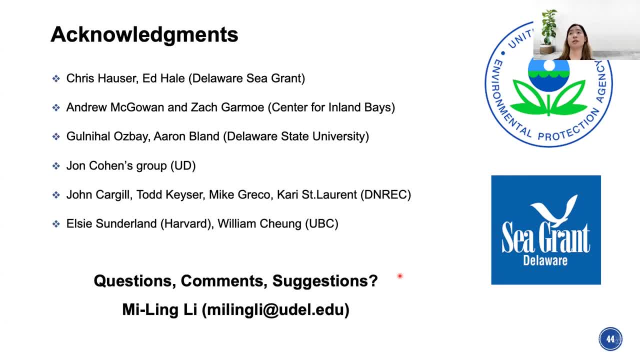 levels, Because that's mercury and PCB- are monitored, And that's why they're monitored by most of the state's government. So we've had a lot of questions online about mercury. But, Mimi, we'll start with a few, Okay. 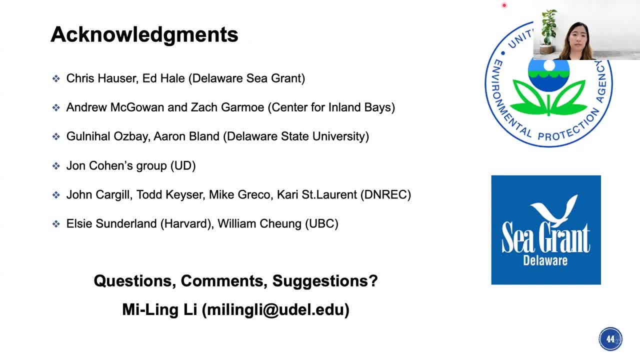 Yeah, I can work very exactly. Actually two, No, just two minutes. So Rene Altmaier wants to know: how are they making it possible for less than a part of the trillion concentration to be measured and controlled by the mercury? What are the downsides to that? 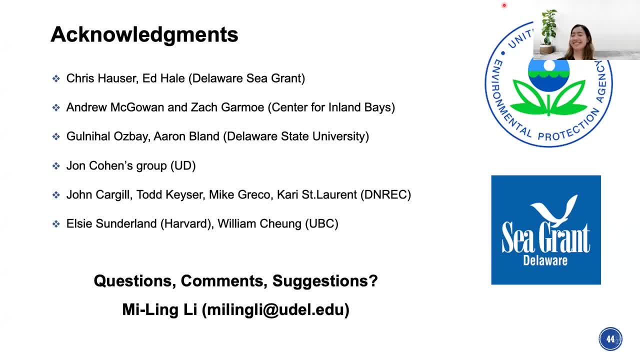 And what can we do to prevent that? And so I think that's a great question. So the first one is: I think in the last two years we've been doing a lot of research on mercury And we're working with some organizations, I think for a long time, and it's been 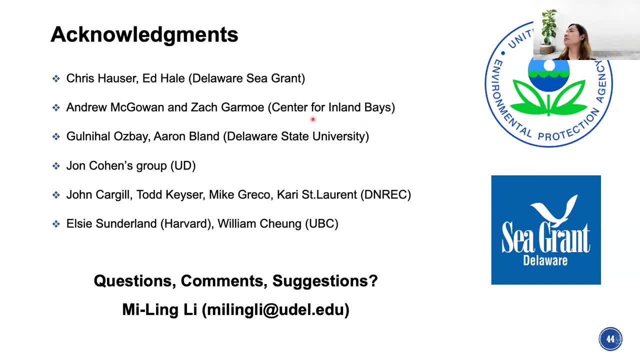 a lot of work. So reading Altmaier once in a while, how I would say, is it possible for less than a part of the trillion concentration to be measured and controlled? Is that a useful number? If the limit is 0.004 ppt, is there any way to detect and do anything about levels that low? 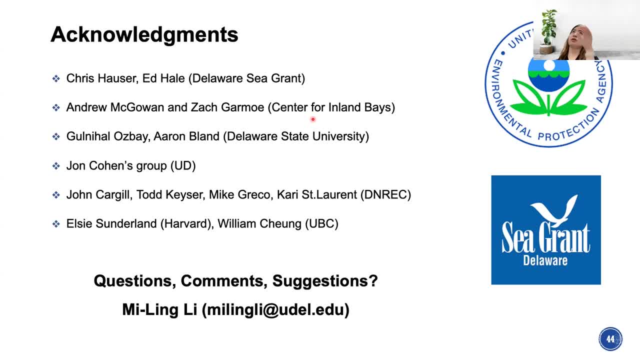 Yeah, so far based on the EPA methods, which is I think you filter 250 ml or 500 ml water and then kind of you enrich them and kind of measure the concentration For lower than 1 ppt level. I think for most of the instruments you know over the world are not that sensitive. 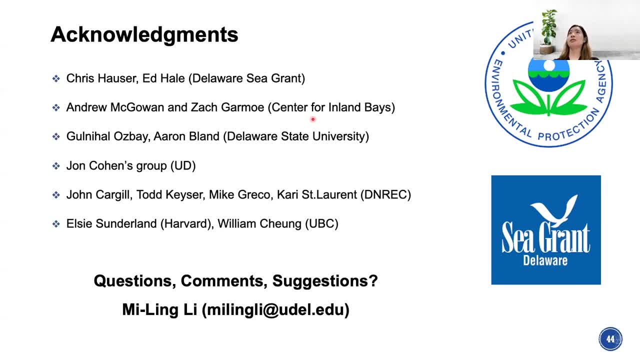 Yeah, so I just want to stress that that helps, And I think that this advisory is simply based on the health effects for protecting health, So they haven't taken into account in terms of regulation feasibility economically, you know, any replacement in the future. 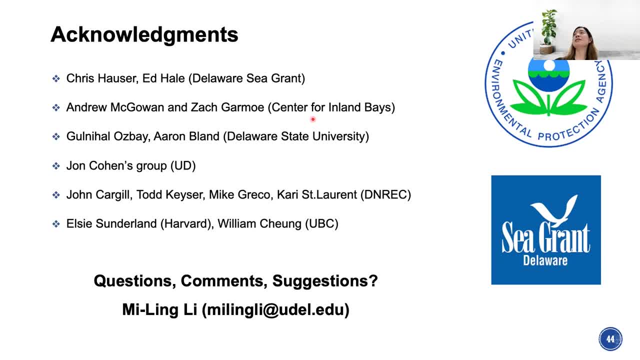 It's. I would always say risk assessment and risk management are two different things And in terms of how we're going to manage it and we'll you know what's, the regulation would be, Because this is a health advisory right. 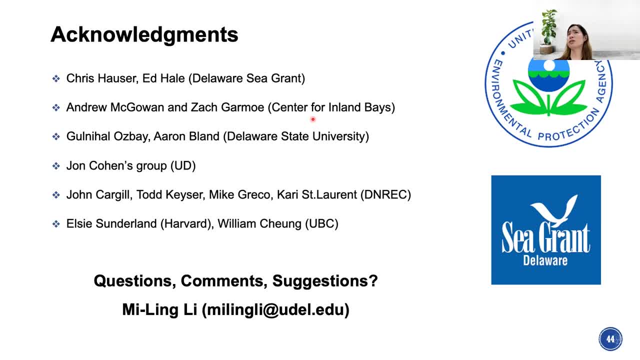 I think that's a question for EPA and I think they are actually have quite bad hearing and information session. that I mean. at least last month I saw one and this month there's an upcoming one. My guess is they try to have this health advisory just let people know this is a safe level, and then they also will have a screening level, which is like we really have to do something. 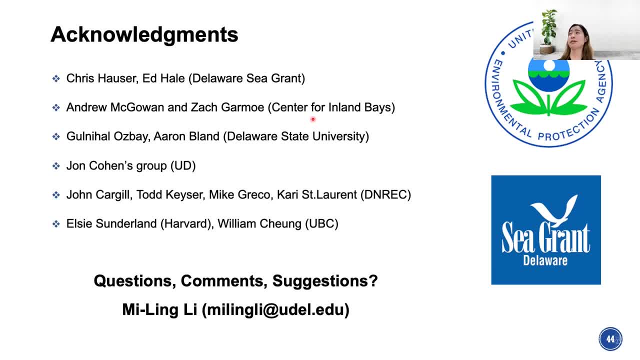 And I haven't known that level yet. I think that probably is coming out as well. But that's a good question. It's basically can detect if that goes gets that low. But I guess, unfortunately, most of the waters now I'm testing it's definitely about the it's detectable. 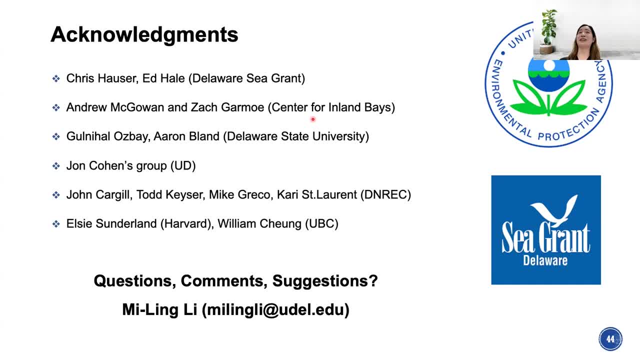 So I don't know if it's a good thing or bad thing. As a scientist, it's a good thing You get a number, but, as you know, as a public it's not really great. Yeah, Yeah, I think that's a good question We have. we'll kind of get some of the mercury questions too. Is there any way to filter these contaminants? Is there a way to remove what is in the water? 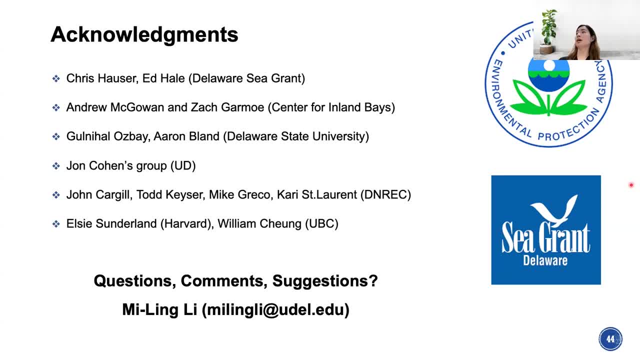 Yeah, So as an end user, household the RO system, the remote osmosis system or just even just carbon filter. you can't get all of them out, but it's quite efficient. Yeah, So you can do that. I think I would recommend, if you suspect your water. 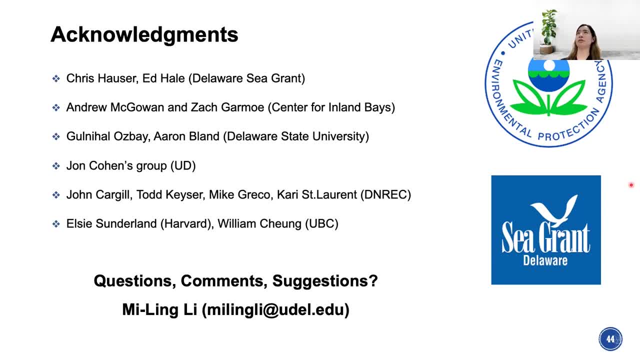 Right, it's, you know, kind of contaminated, or we kind of worry about your water. I I would suggest filter it, And most of filtration system actually could work. The difficult part is water in the ocean, No water in the natural ecosystem. What can we do with it? That's something I think lots of scientists are thinking about that a lot. Yeah, But as a small scale it's doable. 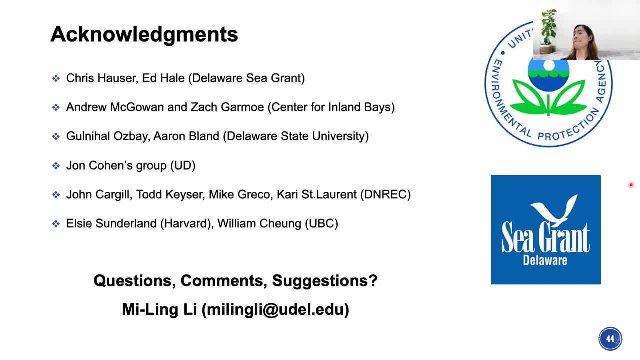 That was one of one of the questions. to switch to mercury. Yeah, Yeah, Yeah, you know. there's a way to remove mercury from the ocean and follow the. you know, regardless of whether or not, is there a way to remove it from food before, 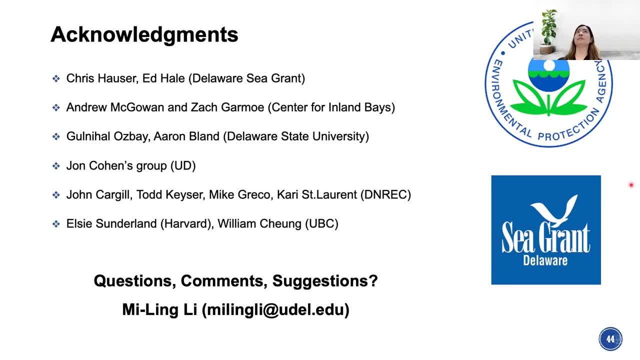 that's a very good question. um, i don't think there's an effective way to remove mercury from food because mercury bound to protein. so unless you don't eat muscle, fish fillet or something, then you can't get rid of them. so pcb is different thing. like pcb they kind of concentrate in the 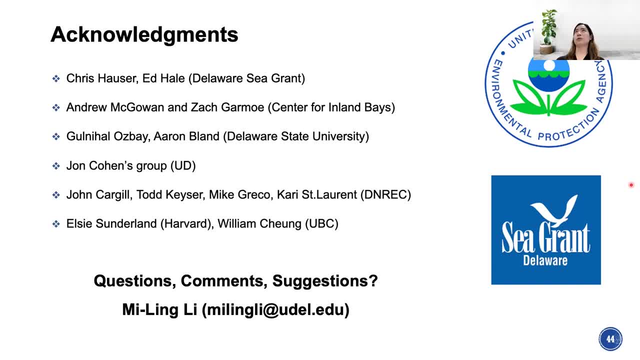 fat. so lots of time. people will suggest if you worry about pcb, you kind of skin off and get the fatty part of mercury, you just can't do anything with it. it's there. it's there, mercury in the ocean, not any engineered way that you can deal with it. i mean heavy metals like basically. just waste until you know. they absorb to biota particles, then they sink to the ocean basin, then over time it's the sediment barrels and they become a deep ocean, you know kind of sediment, and never come back. That takes a really long time. So that's why mercury is so important to cut the emission. 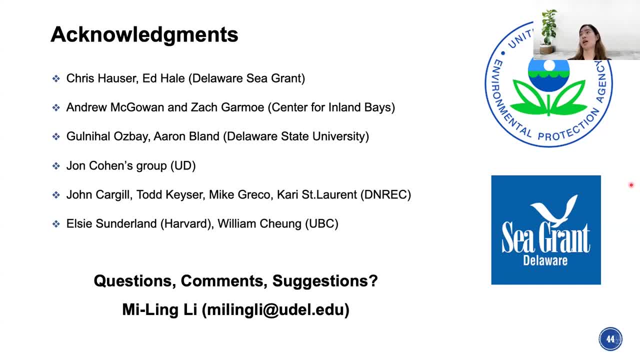 because we just don't really have a very effective way, Although for point sources, co-combustion and these facilities they can. So that's lots of countries- remember we have the treaty- so they install some scrubber to kind of remove mercury, absorb mercury before the air goes. 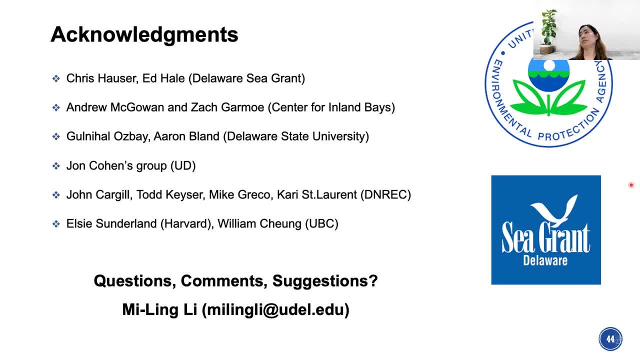 to the atmosphere. Yeah, anybody, just jump in and you guys come up with one. Is there any way to check for mercury in food, So it can't be removed? is there any way to know? That's a good question. Well, I mean, a scientific lab can do that. but 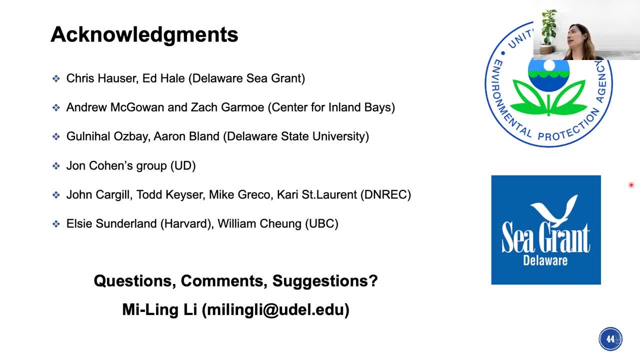 I don't think normally like any industrial like yeah, it's not something I feel like you go to a store or something that they would tell you that I can't think of any source of that. But again, I think most of the fish that if you follow the rule of like don't. 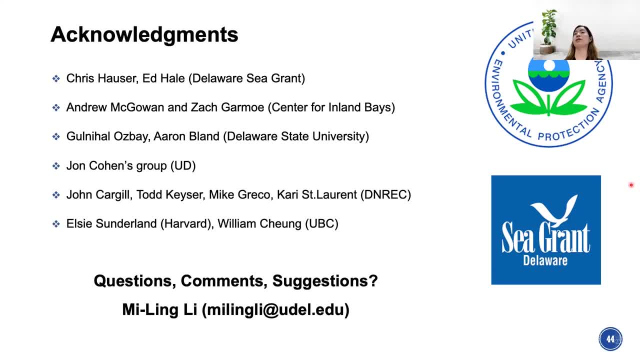 try not to go with this really high trophic level predatory fish and try to follow the fish consumption advisory posted by FDA. it's actually quite predictable in terms of the concentration of mercury in the fish. Yeah, you mentioned that PCB concentration is bad. The mercury concentrates in protein, Yeah, So that's kind of known. 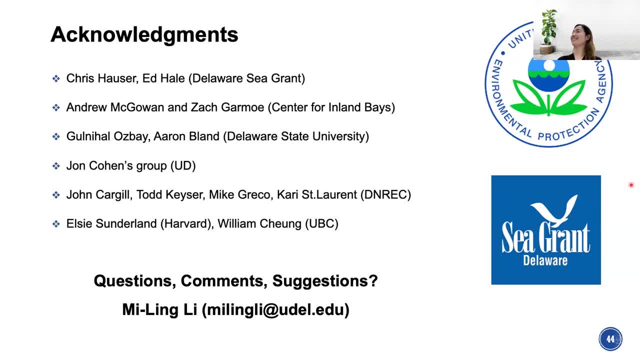 That was a question we had, but just making sure I heard that you had just answered it anyway. Diane asked that question. she also asked if chelation can help with decreasing mercury in foods. Yes, that's one way people does treatment. 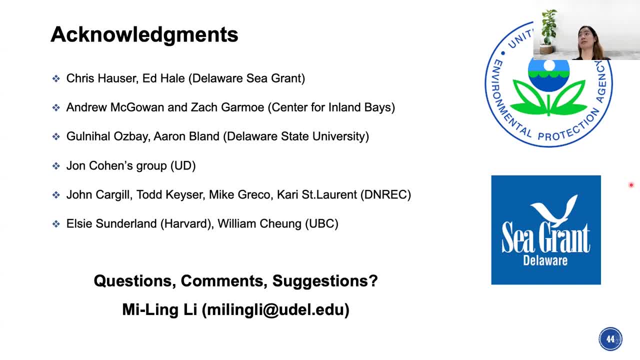 For people who have a really high concentration of mercury in their food blood. usually there's already show some effects. yes, for the rest of us, can you explain chelation? uh, i think it's chelation, so it's i, i, i believe it is something that's like kind of chemicals that. they try to- basically i actually never- i mean i never did that, but i believe it's also like ivy or something. it's like a safe level and they kind of try to bomb the mercury uh from your blood and then kind of get rid of it, um, probably from urine or feces it's uh, so that it doesn't keep. 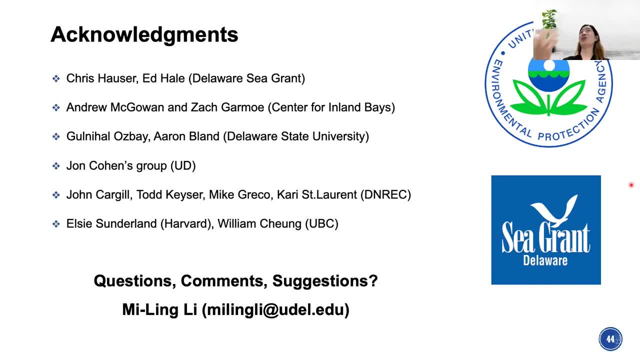 circulating. so basically, kind of you kind of inject something that's the kind of as a, as a binding or absorbent, uh, into your body. yeah, yeah, exactly yeah. but normally i think people, people have very high concentration that they would do it. i know one person- they. is a billionaire and they he eats like sushi every day. it's probably all tuna every day and they keep passing out and they went to hospital and found the, so usually mercury. it's easy way to test. they just tested the hair mercury concentration. that was probably like 50. 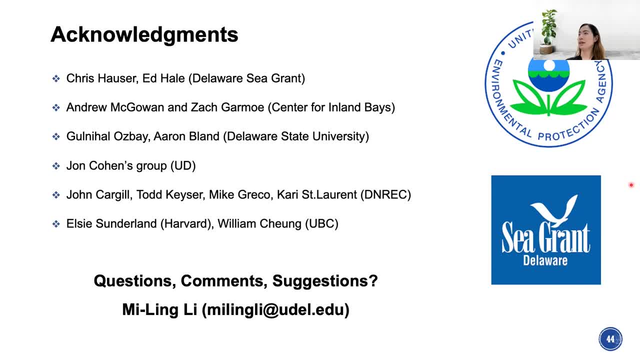 times higher concentration than normal people. then they start the chelation. yeah, um, i think i'll finish diane's list here. um, she had one more. she was asking: is autism related to mercury? i think that might come from the vaccine, the the bones vaccines, but 98, but you know address. 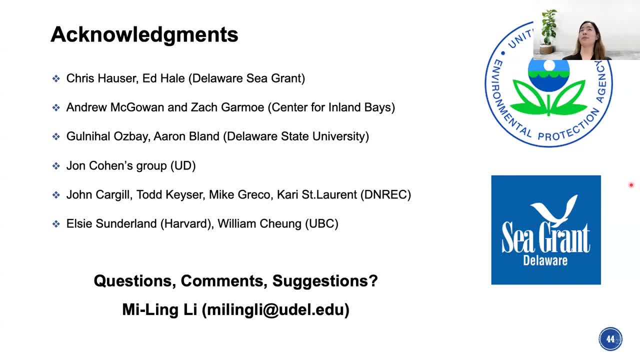 that it's very controversial, um, and i think um. my takeaway is: i, i don't directly do the autism and the mercury study, um, association study, um, my, my takeaway is: um, the, the vaccine or whichever medicine, that, that, um, that has a higher benefit than the, you know, the, the pros, that's way higher than the cons. um and um, i, i think lots of time. 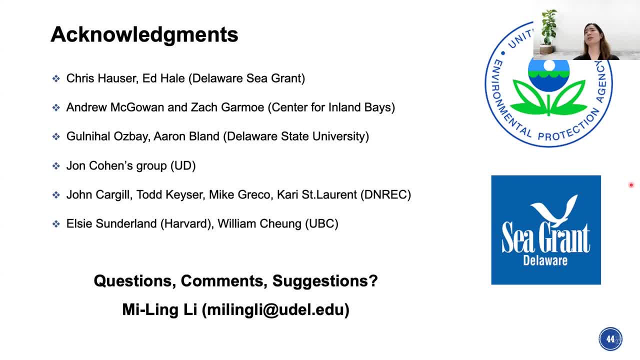 because mercury- now we try to phase out. so i think vaccine less and less vaccine will have mercury first of all, um second, i don't think there is a strong evidence so far that these two are correlated um. so i guess the evidence, maybe one study, show- yes, yes, this study is not so it's like really inconsistent um. so i wouldn't really 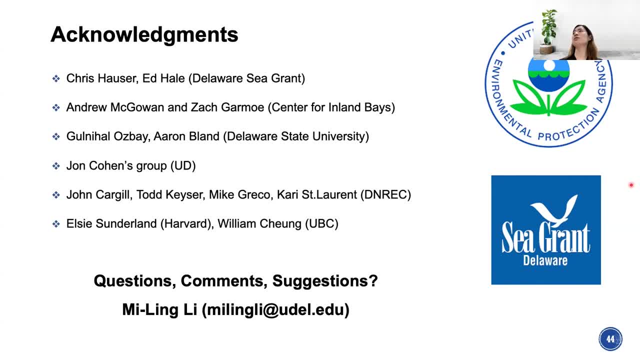 think it's a. you know, i don't prove it's a solid association, um, but i guess everyone can have their own take about that. mercury is known to be a neurotoxic but, not knowing what, you have a relationship with others. that's still being investigated. essentially, exactly, yeah. 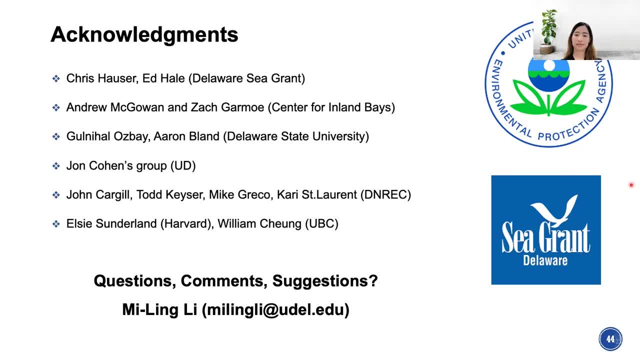 um, there are a lot of practical questions which you would expect in a. you know talk about pollution. um, somebody mentioned from very early on, you know, yeah, that's kind of the example of the millionaire in the sushi. does the marketing level go down? not that much, yeah. so 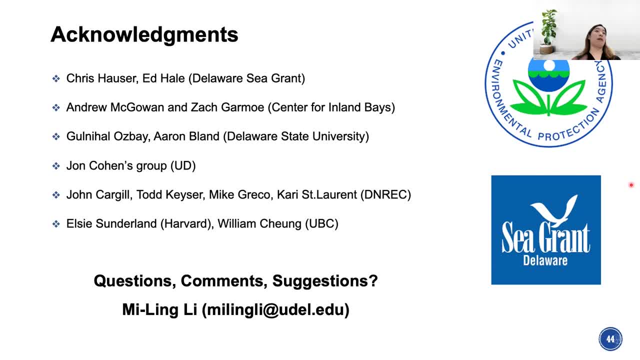 i wish you really stick with the protein. it just people tried, like a grilling, other different cooking methods. people tried with different herb, a different thing. there's no strong evidence that they can remove it there, although that which is really under studied, um is people were saying, maybe after cooking or after certain methods, that the bioavailability which like how much you have. so when you look at the fish, how much mercury is still there, like i don't think that will have any decrease or a significant decrease. but when you eat them they may actually interfere with absorbent or uptake of the from the body. uh, to take the, the mercury, so say you know. 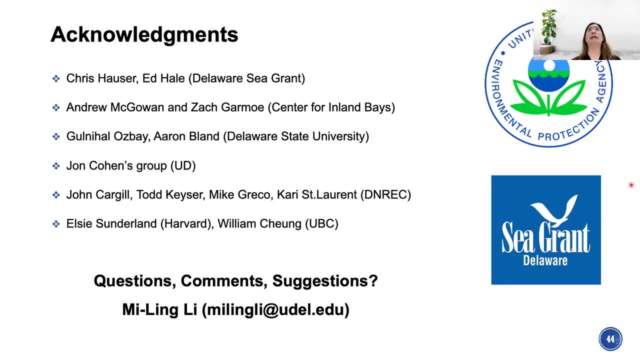 our original mercury was believed to have almost like 98 or 95 percent of absorption rate, which means essentially what you eat or go to blood. but maybe this one can decrease the efficiency. that is totally under investigation, but that's something we're really interested because that 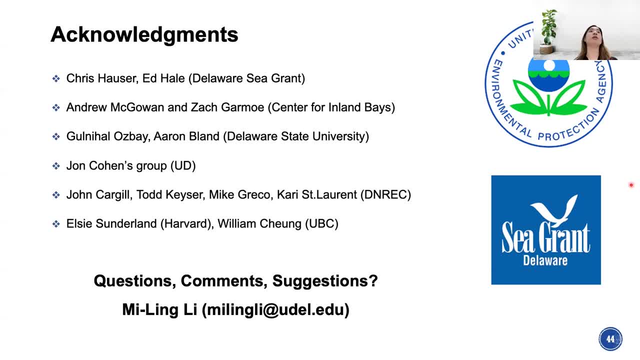 could be kind of prevention or strategies for public health. yeah, somebody online- vivian says she hasn't been the red card box that looks a lot like the one in your slide earlier. um, she's wondering about what kind of danger um that that box or things like that might have. so the box, oh the with the 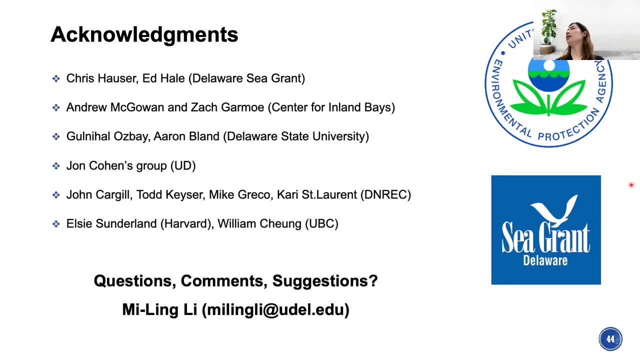 red, you know mercury, the colors that have been, you know it's been used for um. it does depend a lot on how that red is made, but maybe, just generally speaking, how much of a risk is thermal um absorption of mercury? somebody else was asking about um, actually the the mercury in cfl light bulbs, right, cfo, oh yeah, the light bulbs. so if you break your light bulb, how much do you need to worry? right these contact issues. so again, um the the most toxic form of mercury is methylmercury, which is in the seafood normally, the light bulbs ones, and the paint or whichever if they. i don't know. 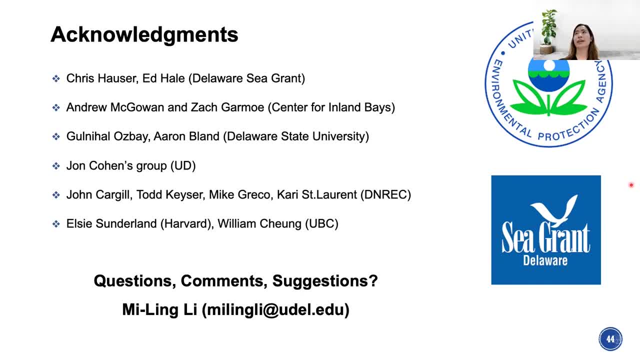 what's the paint made of? if they have mercury, it's likely the inorganic form. so, um, first of all, they they're not that toxic. so don't lick them, don't eat them, for sure. but i wouldn't worry too much about the thermal exposure. um, if you have a light bulb that has mercury inside. um, if you know. 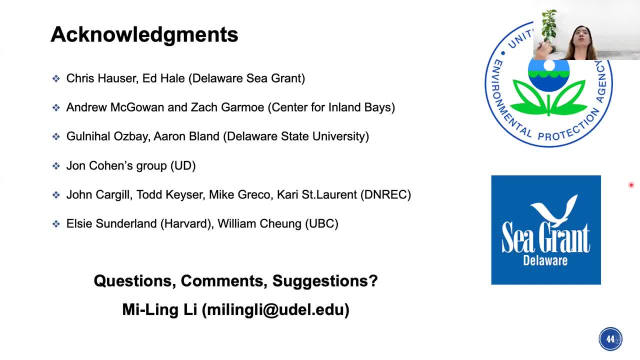 abruptly, just it just broke. then i would just make sure the ventilation is going on. um, then it disposed them. um, i wouldn't worry too much about inhalation as well in that case. um, and the uh the thing usually as a scientist we worry about, you know, about the, say, red chips. so 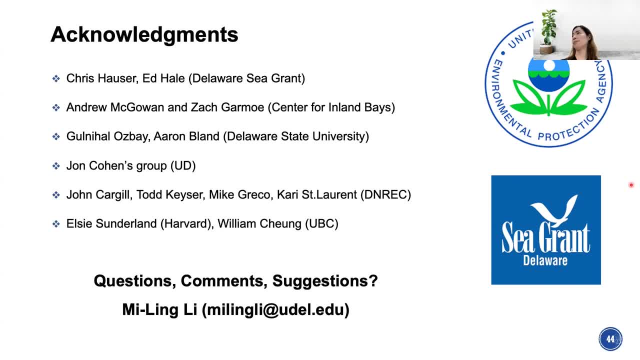 containing paint, containing mercury or other things containing mercury, even as inorganic as how i recycled, will that be, you know? going back to the environment, so that's something i feel like i would be more worried about for the environment, not that much, i think, for the human health perspective. yeah, 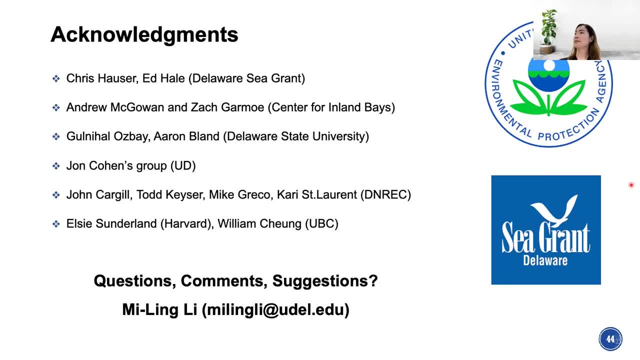 um, it's, it's five after, but only a couple more questions. sure, yeah, go ahead. um. two questions about where else mercury can be found. well, you mentioned it's in the atmosphere, but i think they're asking about is it maybe lower in the atmosphere? um, and then wondering. 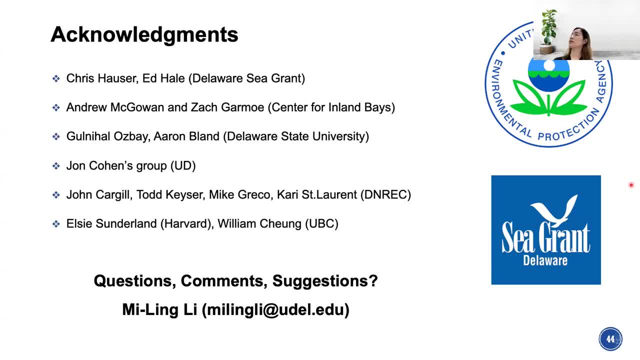 if it shows up in snow, do you say it can precipitate without? yes, so so, if you like, in the rain, in the snow, yes, i mean you can test that in seawater. but um, these are inorganic form and usually very low concentration. that's, it's really. 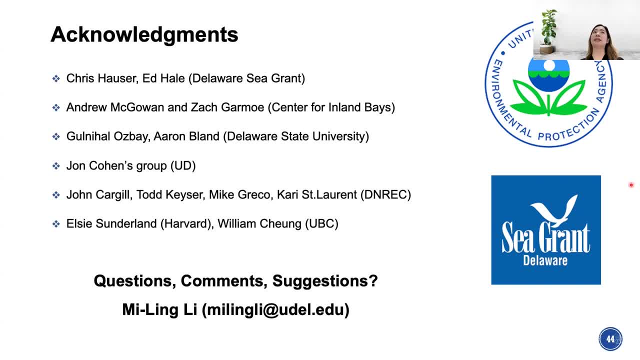 they have to go up to the food chain and go you know a million times higher than let's get something worried. yeah and um, the last question was actually one of the first ones to come in. i haven't given it to you yet because i'm not quite sure how it fits in, but it was about your early. 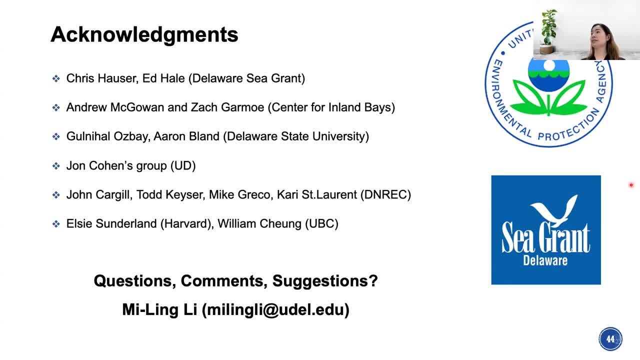 slide about um metals in the body. you know, when you get your body, you you kind of made it just out- ones that are essential. yeah, they're asking about um lead. is that on the list, i guess? yeah, as non-essential. yeah, so they're asking, you know, isn't that very toxic, which it is? so that was. 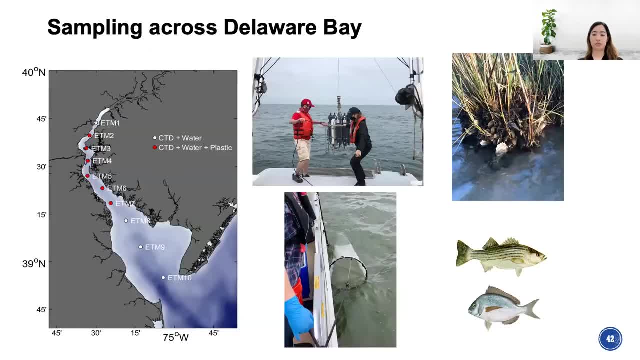 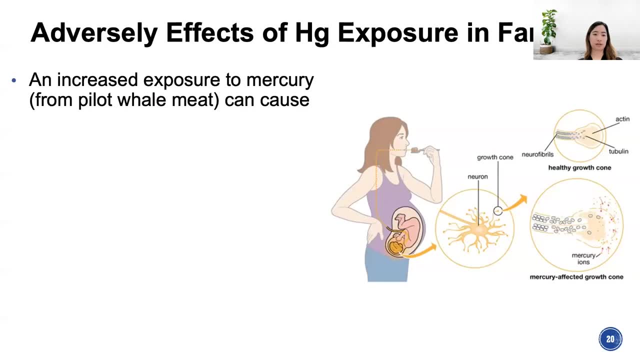 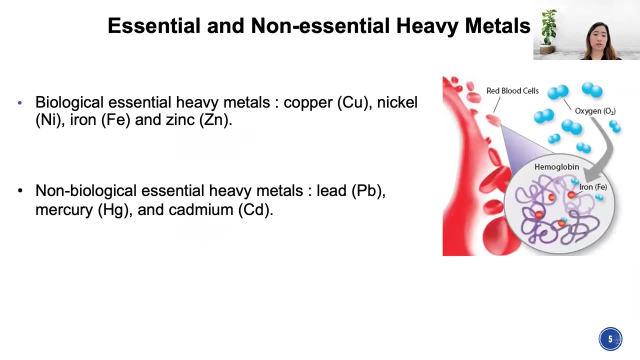 your point right, the essential ones we use in our body, the non-essential ones, including mercury, yeah, so well, i guess that's all the way. i think it's really early. well, so, yeah, so, um, that's a good catch. um, i didn't go into detail about this, um, but yes, so cadmium, that are they both toxic and especially? 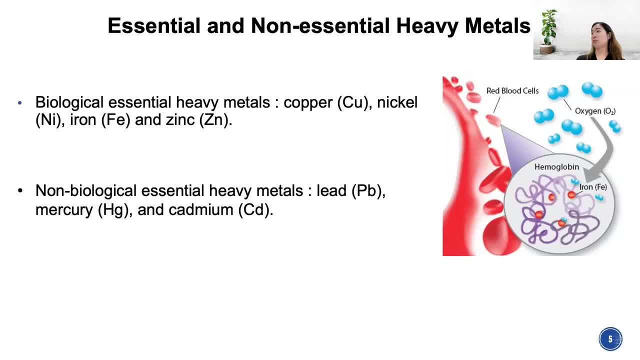 lead. i think you probably hear from flint drinking water issue, all these things, i mean, i'm still ongoing. that is also um widely used in the paint. um, because it's red as well, right, so, um, it's um lead. i would be more worried about drinking water. that's the main source.